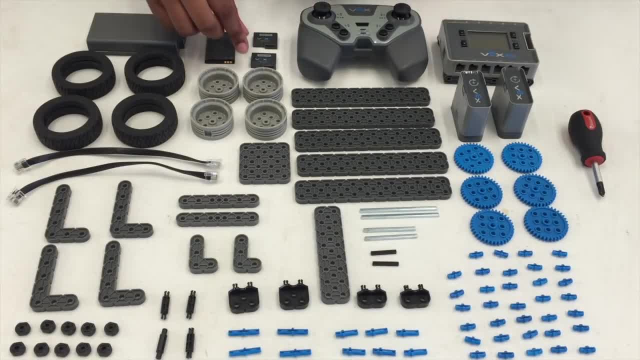 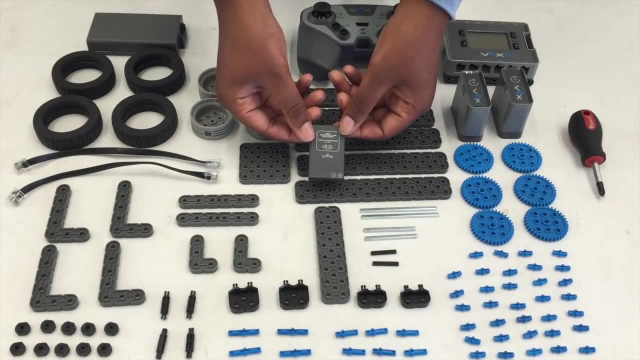 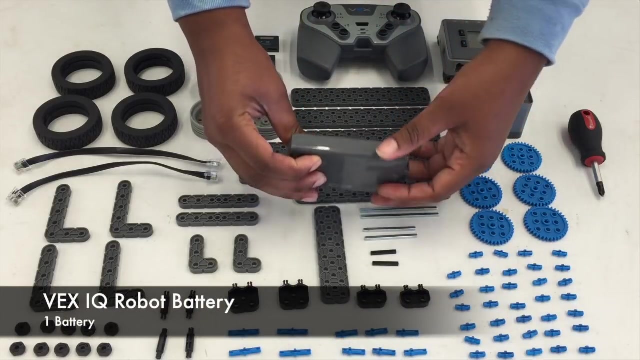 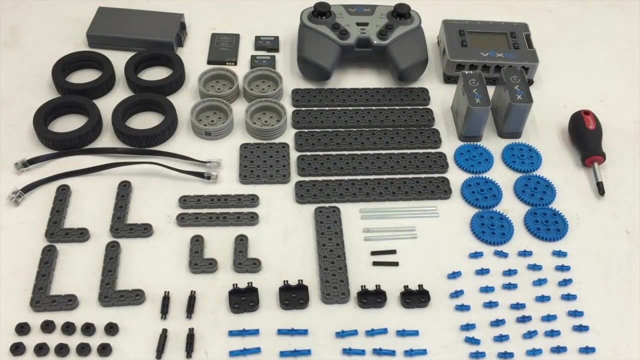 One VEX IQ controller, Two VEX IQ radials, One VEX IQ controller battery and one VEX IQ robot battery. You also will need a partner for this activity. One partner will be partner A and the other will be partner B. 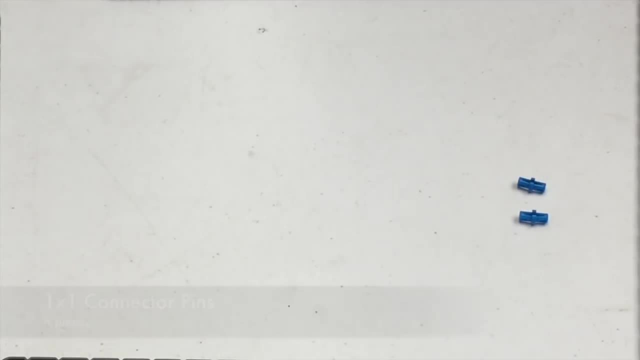 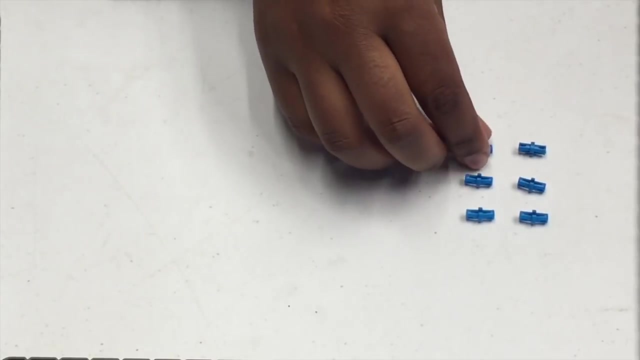 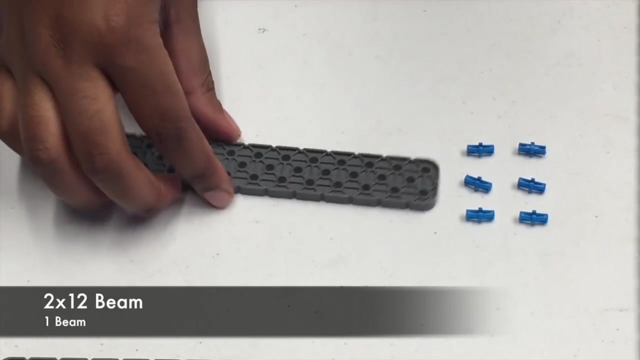 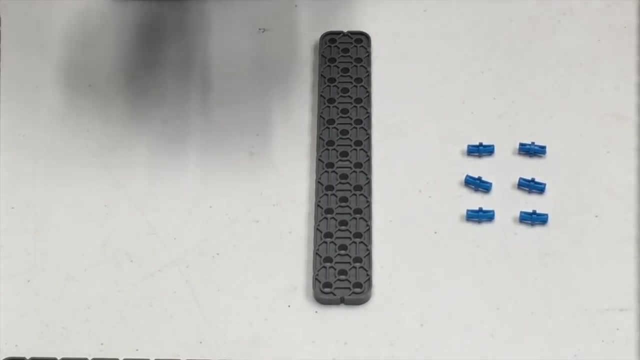 Step one, partner A and partner B will need to each get six 1x1 connector pins. We also need partner A and B to grab one 2x12 beam. And again partner A and partner B in the group grab one 2x12 beam. 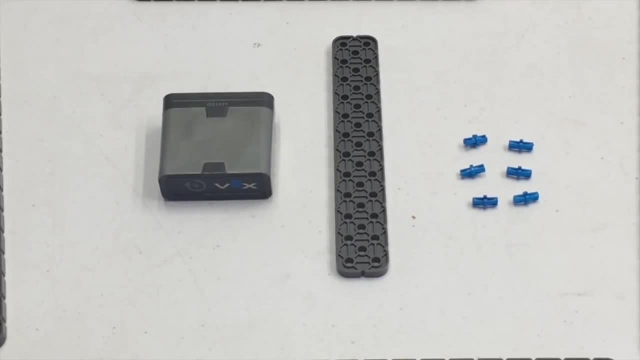 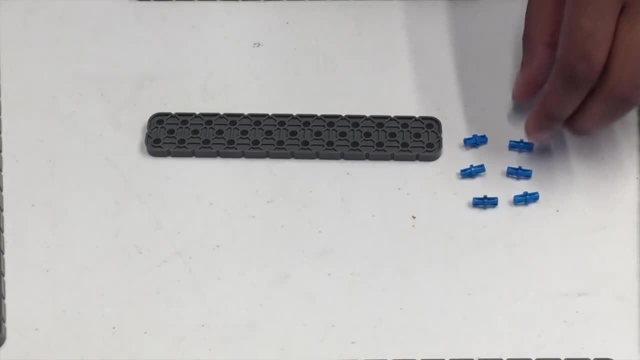 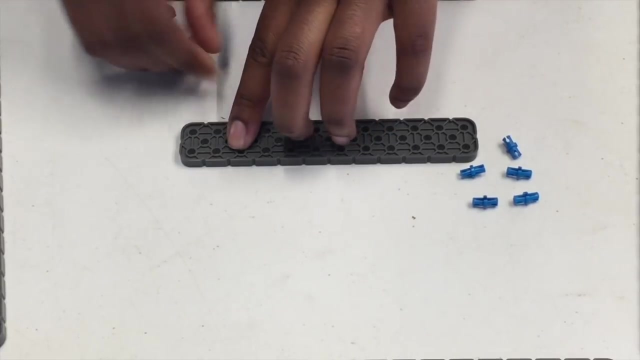 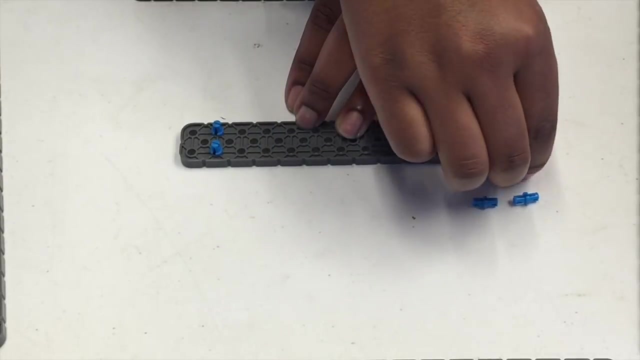 VEX IQ smart motor. Now let's set our smart motor off to the side for a sec And we want to grab our first 1x1 pin connector and skip over the first hole and go to the second hole And just snap those right in place. 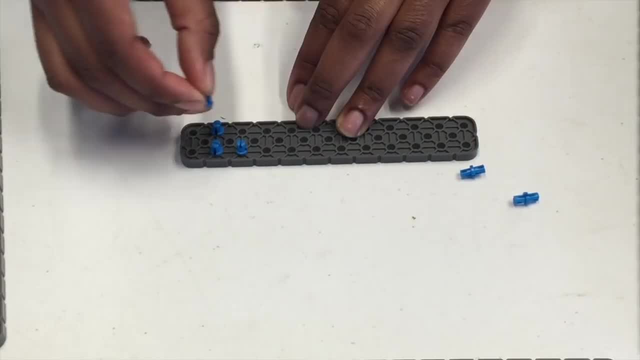 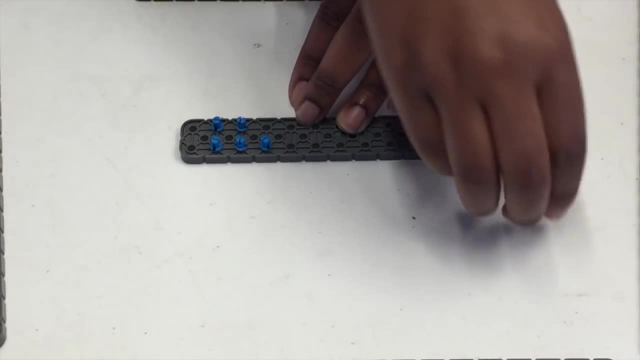 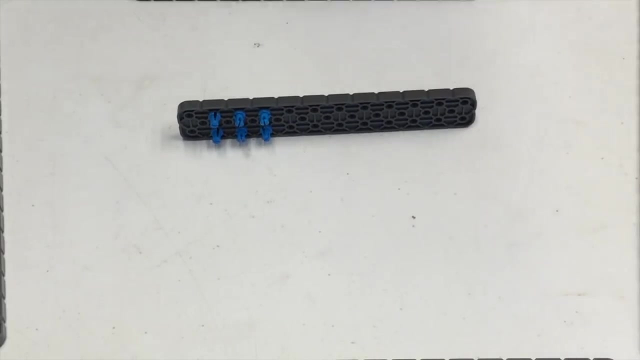 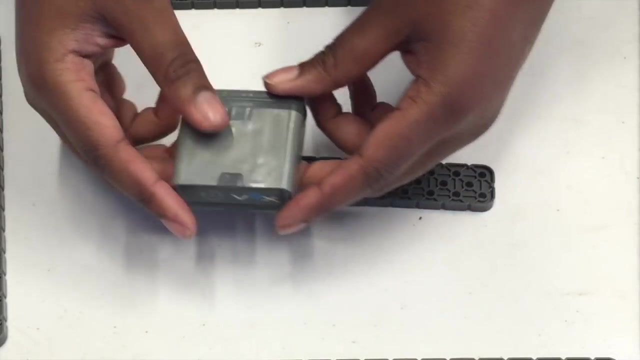 And push all the way down until you hear a click. That's the fourth, one, fifth and now we have all six pins in our 2x12 beam. Now I'm going to go ahead and lay my beam back down flat and grab my VEX IQ smart motor. 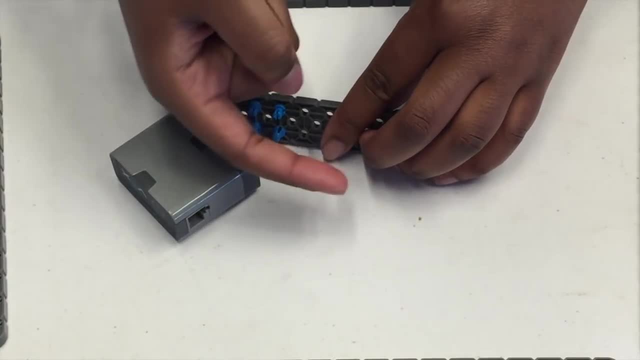 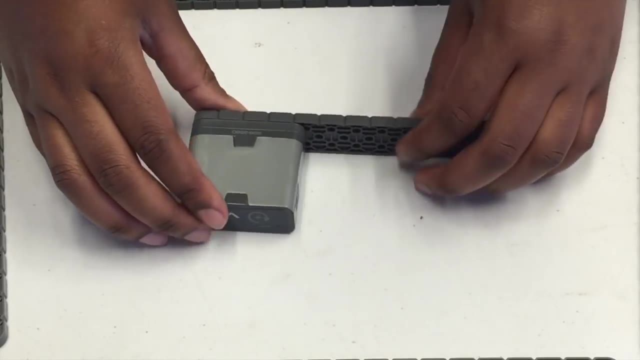 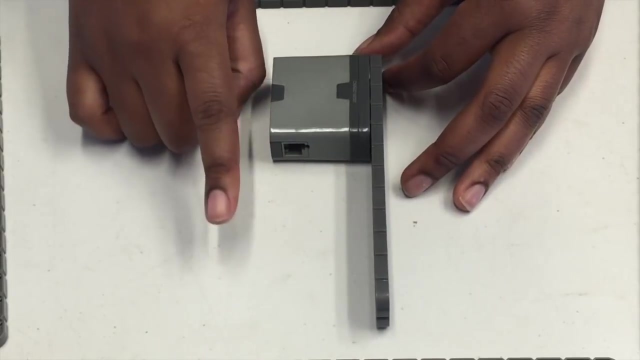 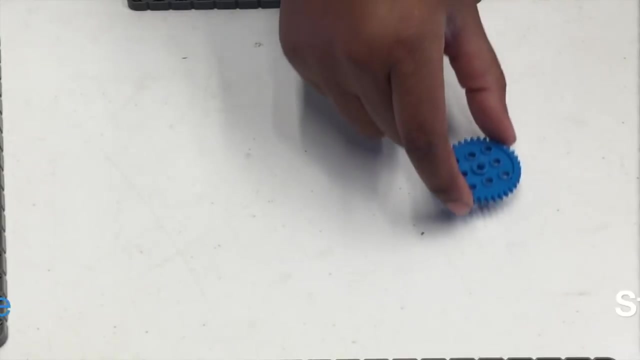 And I'm going to make sure that the opening is facing down the beam And line those two up And just snap them together. Again, make sure that the opening is facing down your beam. So now you should have partner A and partner B with a smart motor connected to a 2x12 beam. 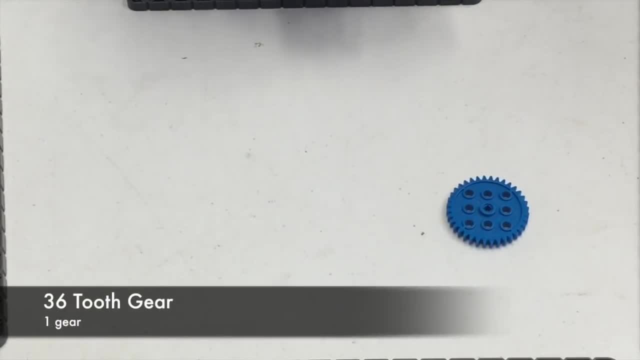 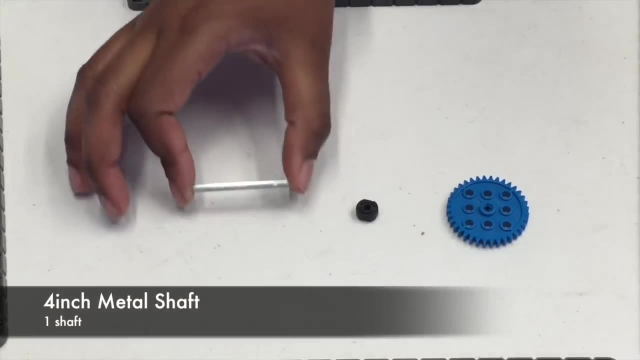 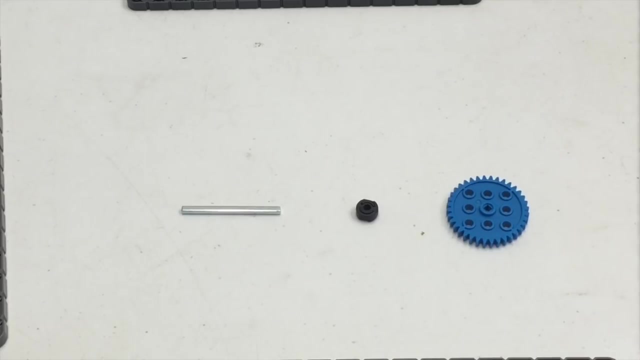 Now on to step two. Partner A and B will need to grab one 36 tooth gear, One shaft collar And one 4 inch pin And one 4 inch metal shaft. Now both partners go ahead and grab that motor that you attached to the beam. 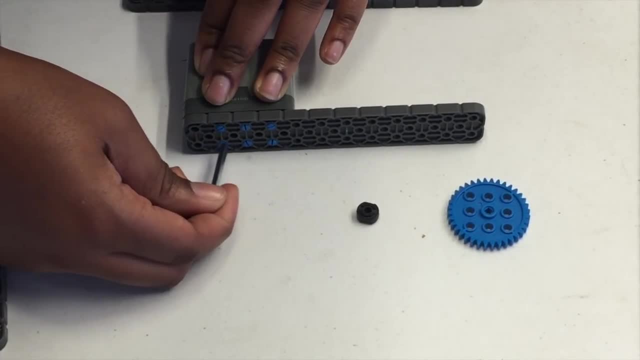 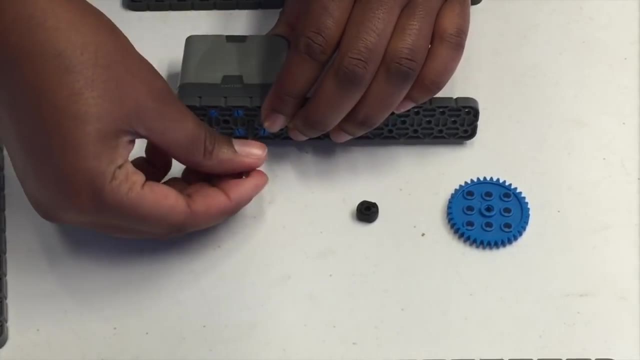 And first we're going to pick up our 4 inch metal shaft and we're going to count out three holes And then we're going to push the metal shaft right through that third hole. Be sure to take your time and line the shaft up with the hole. 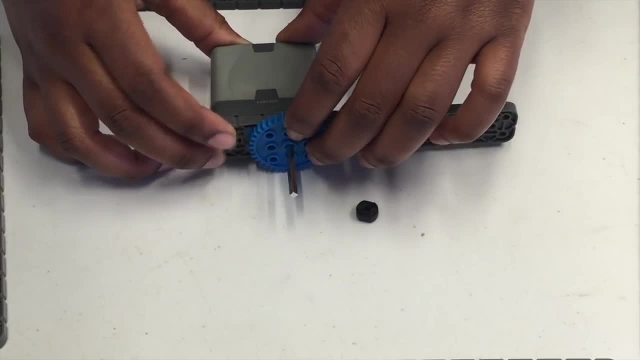 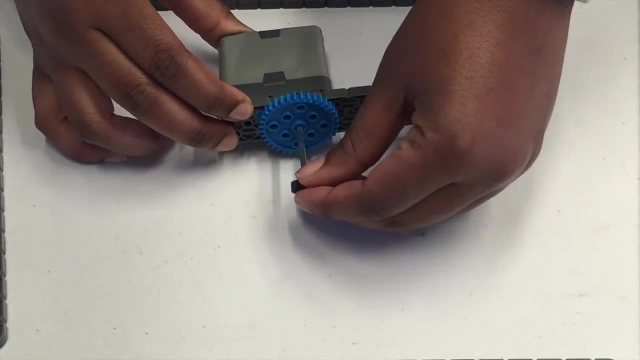 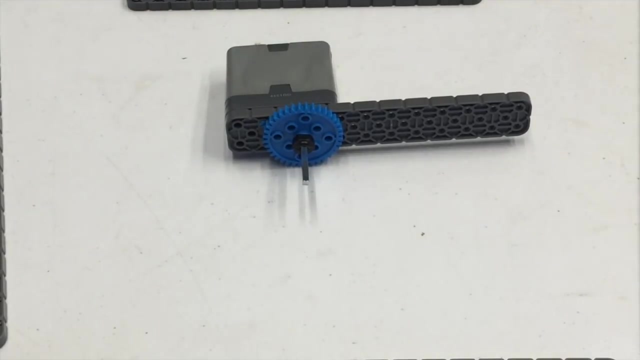 Then we're going to grab our 36 tooth gear and we're going to slide that down the shaft, Give it a tug, Make sure you hear the nice gear noise, And then grab your shaft collar and put that on top of your gear. 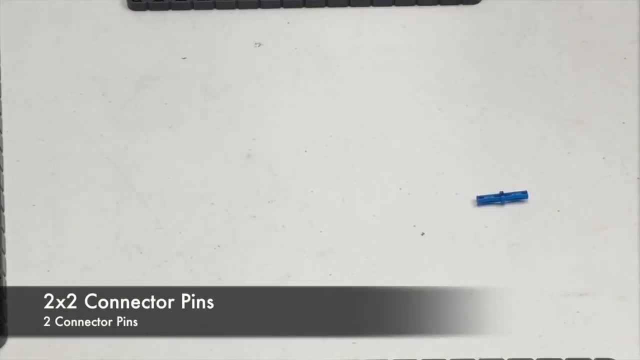 Now on to step three. You will need two 2x2 connector pins And two 2x2 connector pins And two 2x2 connector pins And two 2x2 connector pins. These are the longest one in your set. 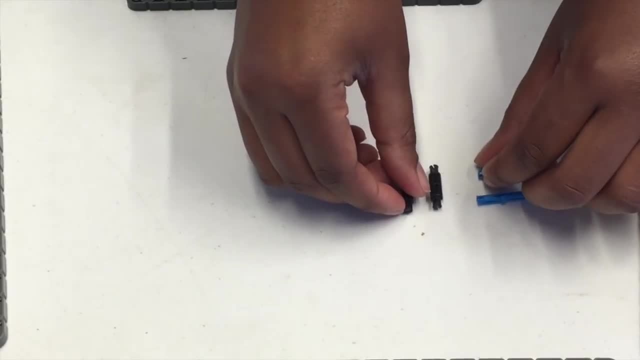 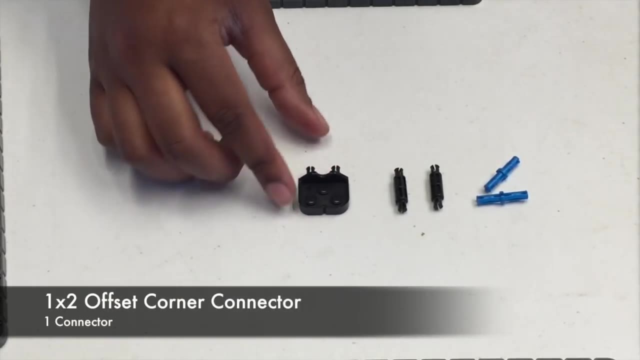 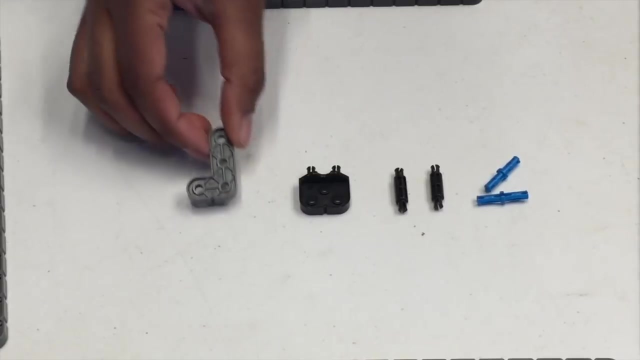 Two 1 inch standoffs- Again, partner A and B is doing this at the same time- One 1x2 offset connector- And notice that the holes are shaped in a triangle- And one 2x3 right angle beam And one 2x3 right angle beam. 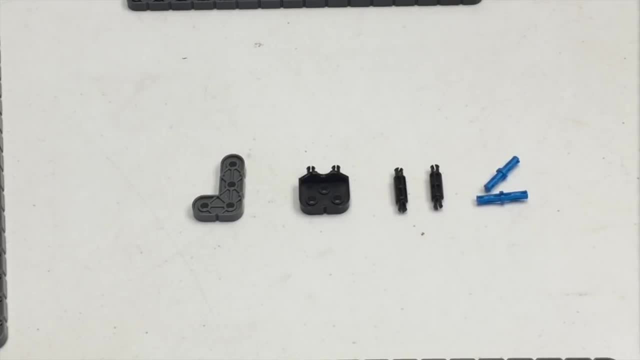 And notice that the holes are shaped in a triangle, And one 2x3 right angle beam And notice that the holes are shaped in a triangle. Take this time to get all the materials, and now let's bring in the motor beam that we 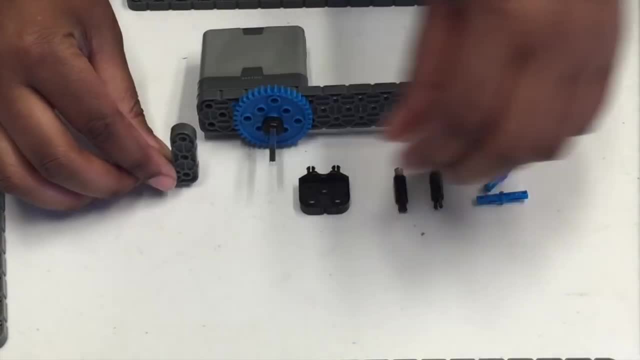 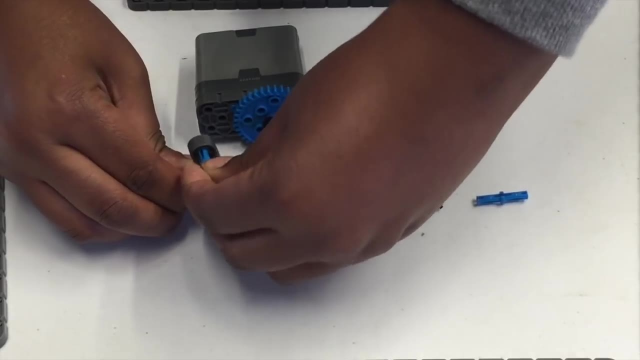 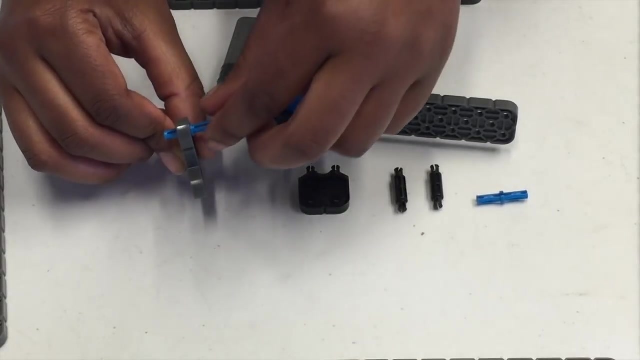 attached in step two. First, we're going to pick up our right angle beam and our two by two connector and put the two by two connector in the top hole. Be sure to push it all the way through so that it's sticking out on both sides. 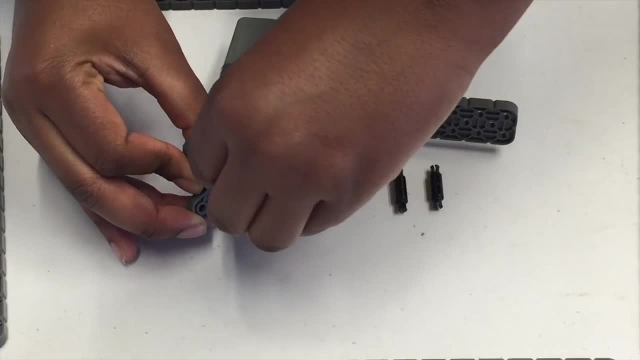 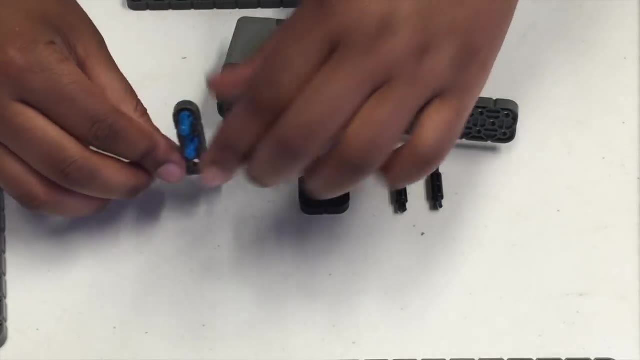 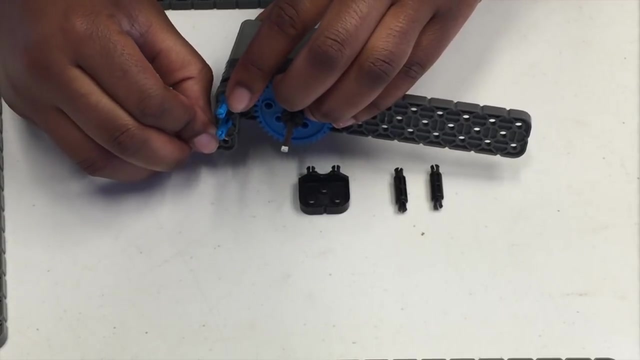 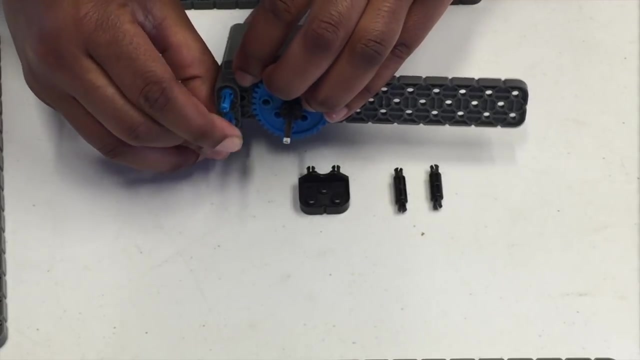 Grab your second pin connector and do the same thing right underneath the first one. Again, push it all the way through so that it's sticking out on both sides. Now go to your motor and attach it at the last two holes on the two by twelve beam. 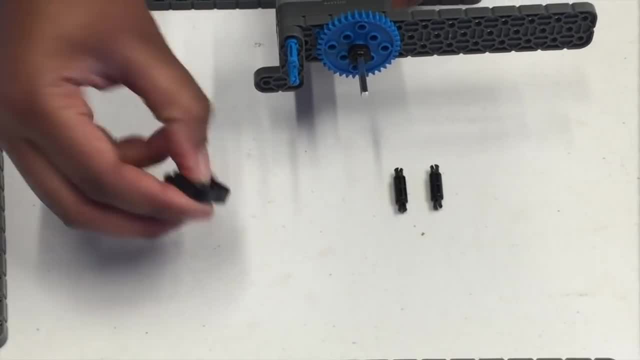 Now grab your all the way through pin connector and put the two by two connector in the top hole. Grab your second pin connector and do the same thing right underneath the first one. Grab your offset corner connector and make sure that the pins are sticking away from. 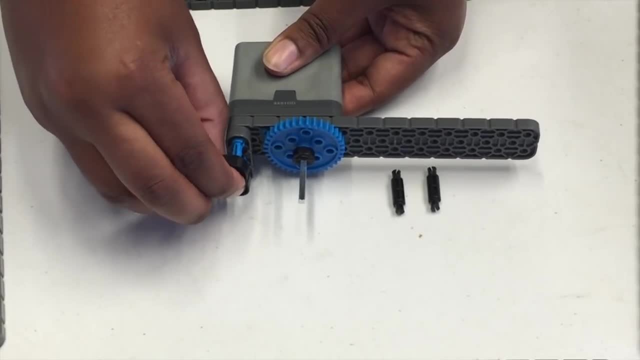 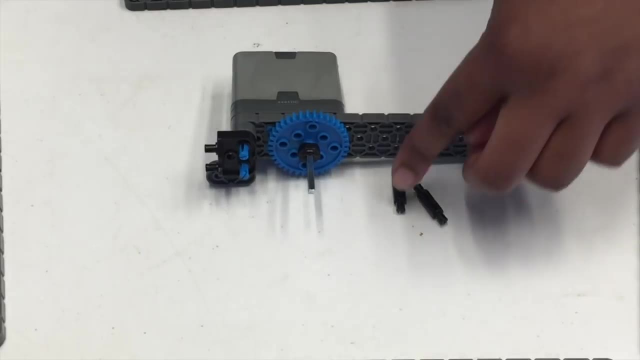 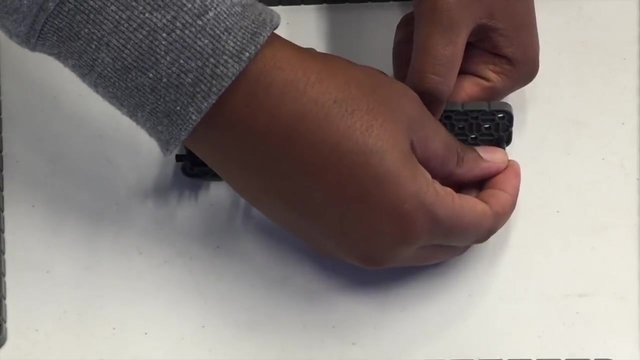 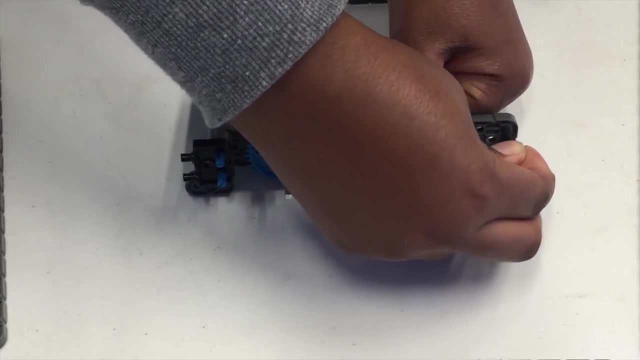 the motor and sticking out the opposite end of the beam and connect those to the end of the pin connector. Now grab your two standoffs and go to the opposite end of the beam and put both of those in the last two holes at the end of your 2x12 beam. 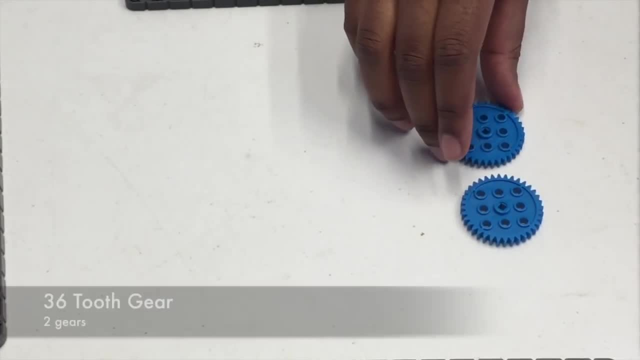 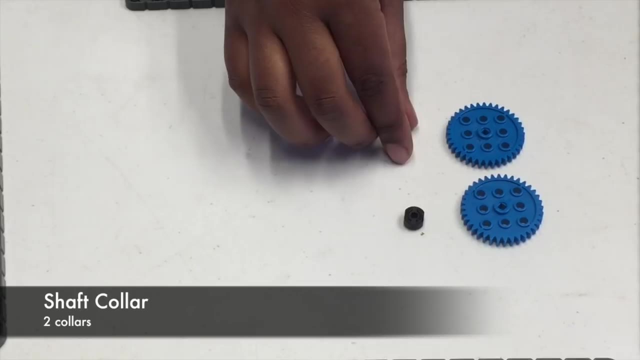 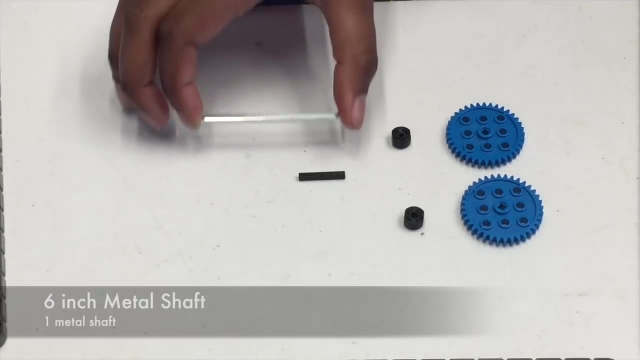 Now time for step four. Partner A and B will need to grab two 36-tooth gears, two shaft collars, one 2-inch plastic shaft- make sure it's the plastic one, not the metal one- and one 6-inch metal shaft. 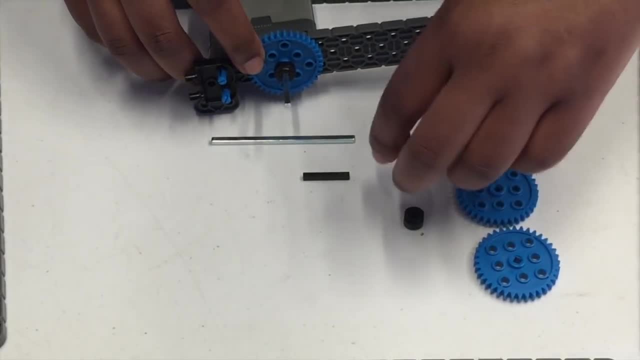 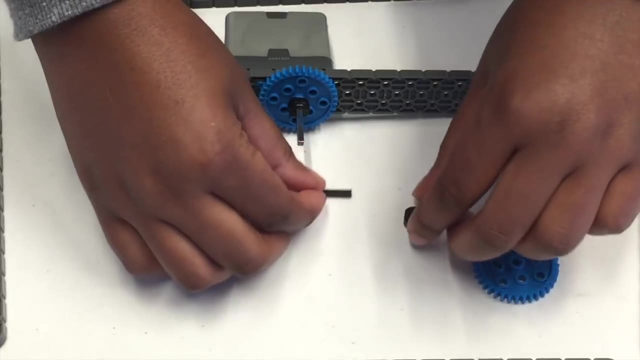 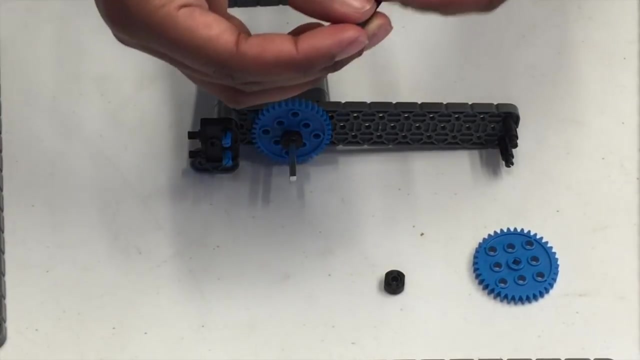 Now bring your gear and beam back into the picture and remove one of the gears, the metal shaft and one of the collars. Now grab your 2-inch plastic shaft and count to the second hole and put your plastic shaft right through the middle. 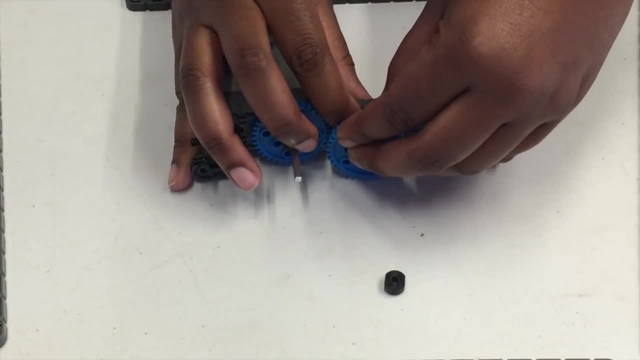 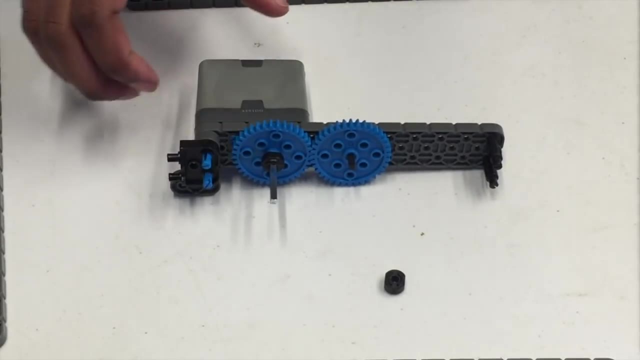 Now grab your gear and place your gear on top of that shaft, Push it all the way down until it comes through. Now you can grab your collar and put your gear on top of that shaft And put that on top and push that through as well. 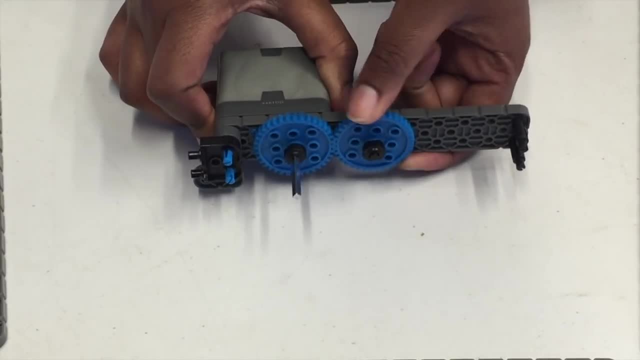 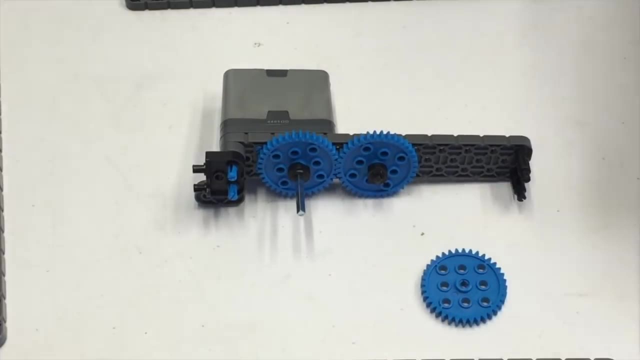 Now you want to grab your gear and make sure you hear that gear noise again. Keep turning it until you hear it. And now we're ready to get our second gear and also grab the shaft- the 6-inch metal one, and the shaft collar. 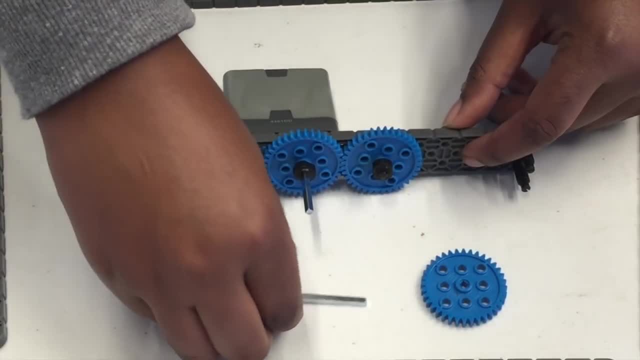 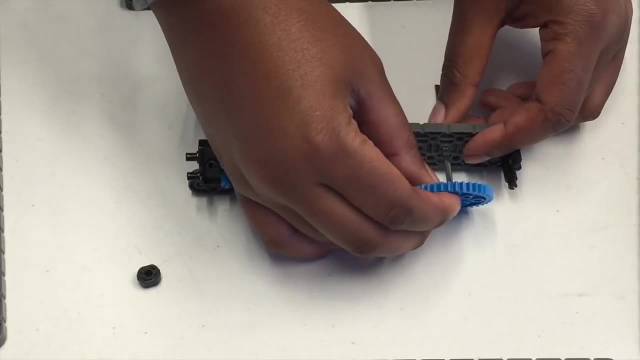 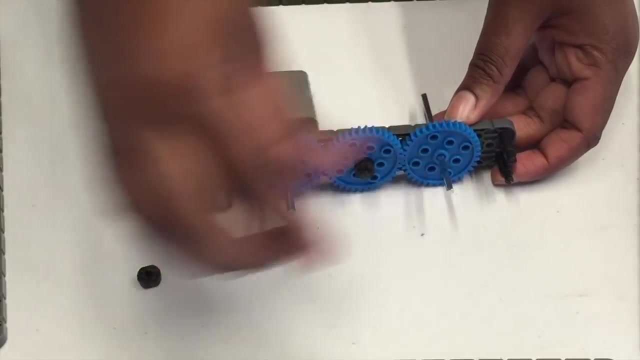 And we're going to count out another two holes. Go ahead and pick up that 6-inch metal shaft and push that all the way through. Grab your gear, Slide that on top And then go ahead and grab the shaft collar and put that on top of the gear. 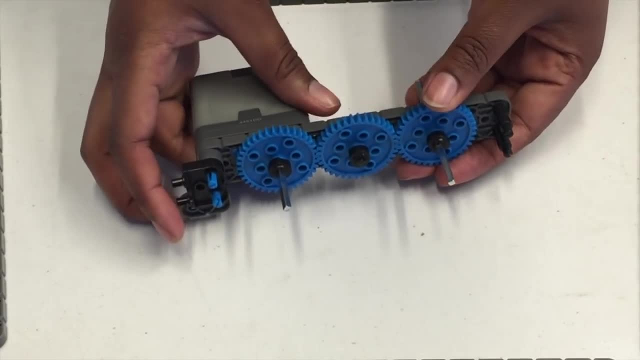 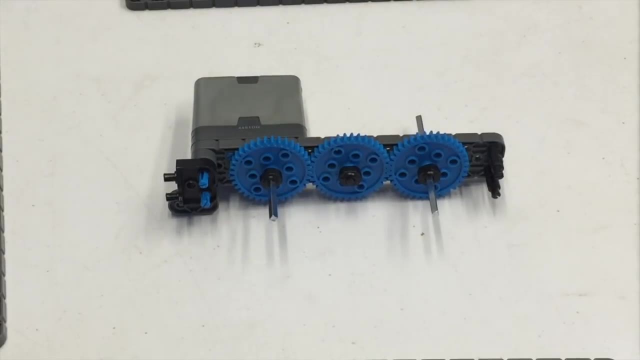 Now you'll notice that your shaft is sticking out some, and that's perfectly fine, And the reason why I'm doing that is because I want to make sure that my gear is sticking out. And the reason why we keep twisting the gear is just to make sure nothing fell out. 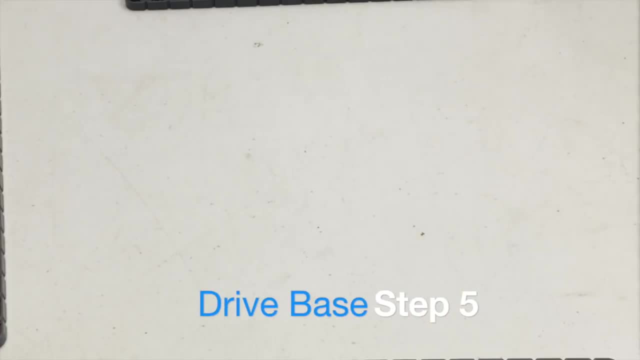 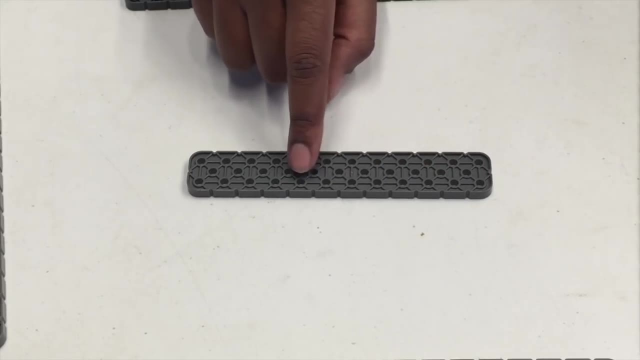 So now we can move on to step five For step five. grab your 2x12 beam Again. this is partner A and B doing this And you want to count them out and make sure you have a 2x12.. 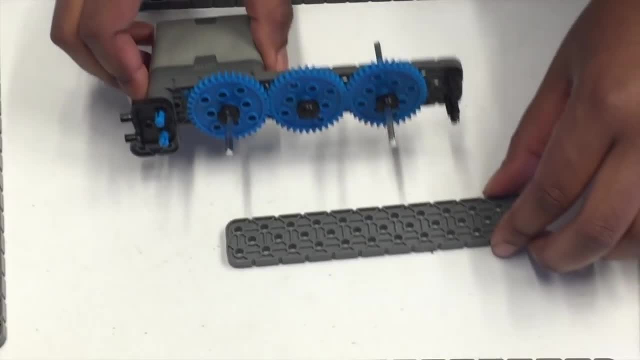 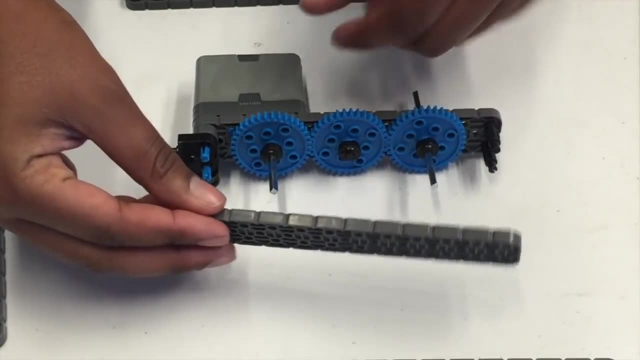 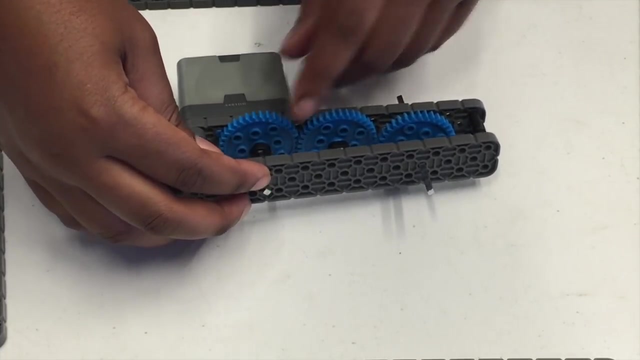 Go ahead and grab your gear that you just made. Go ahead and grab your gear that you just made, And step four, And step four- And pick up your 2x12 beam and place it directly on top of your gears. And place it directly on top of your gears. 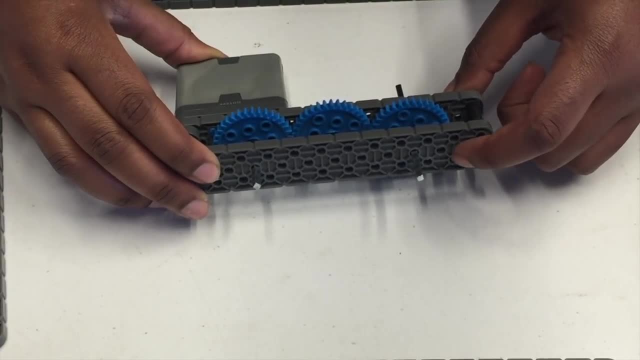 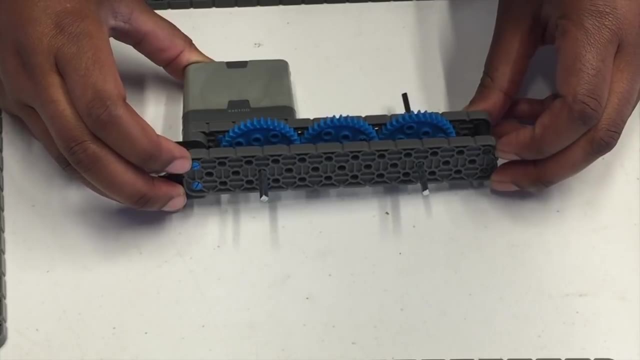 Notice that I am in the third hole. So I counted one, two, three from one end, One, two, three from the other end, And then I snapped it all the way down. Okay, by now partner A and B in the game are in the game. 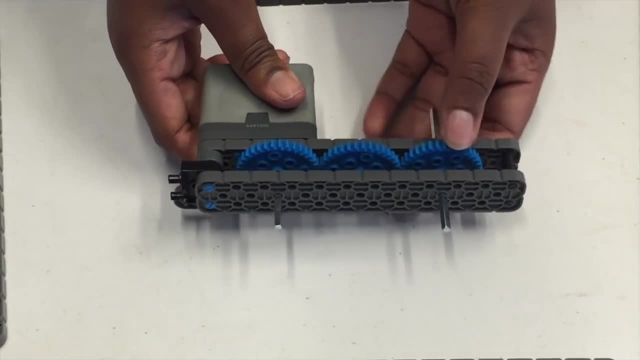 Okay, by now partner A and B in the game are in the game. Okay, by now partner A and B in the game are in the game. You should have two gear box completed. You should have two gear box completed. Now time for step six. 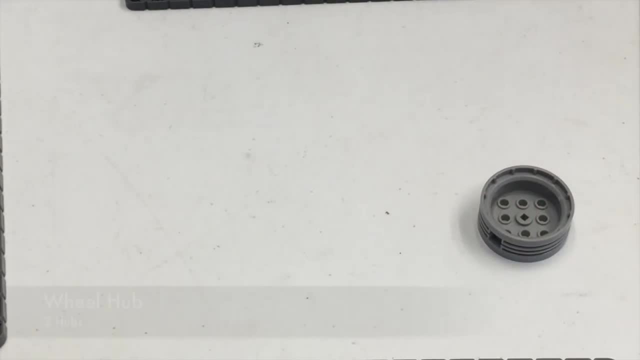 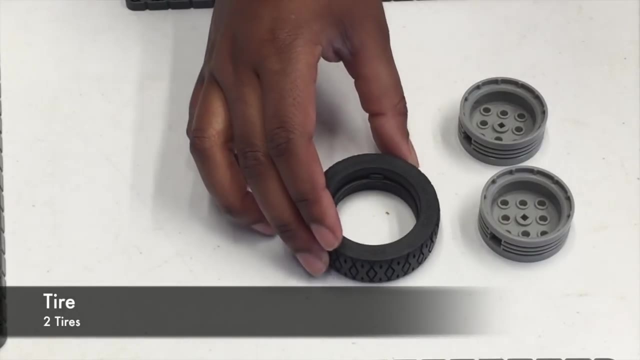 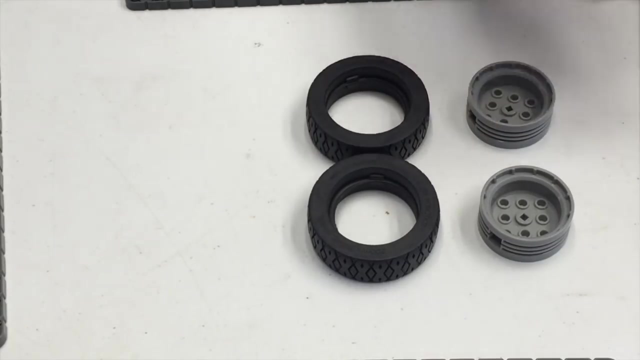 Now time for step six. Partner A and B will need to grab. Partner A and B will need to grab two wheel hubs, two tires and two shaft collars. Now, first, let's take away one tire, one shaft collar and one wheel hub and leave. 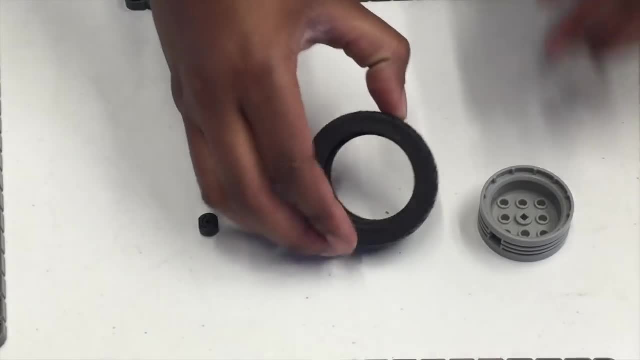 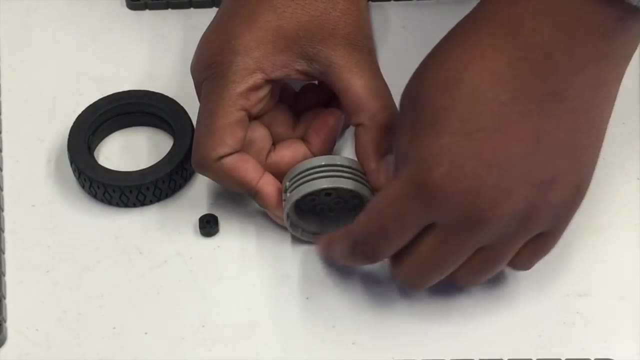 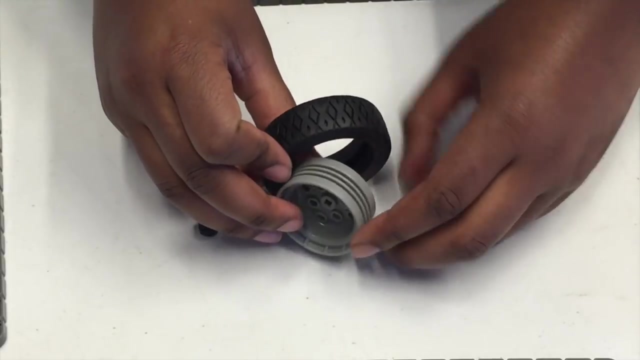 one in front of us on the table. Now grab the wheel hub and first we want to make sure that the hollow part is facing out. If you look onto the tires, they have words on it and we want the hollow part facing out towards the words on the tire. 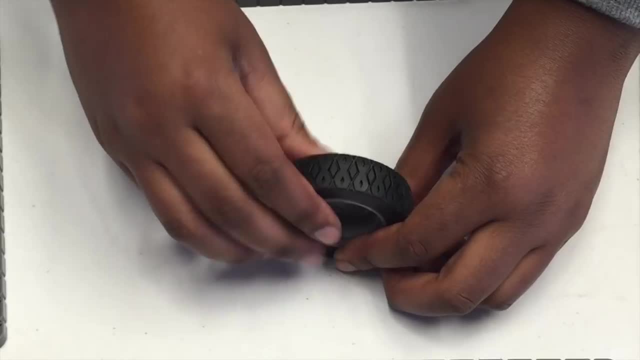 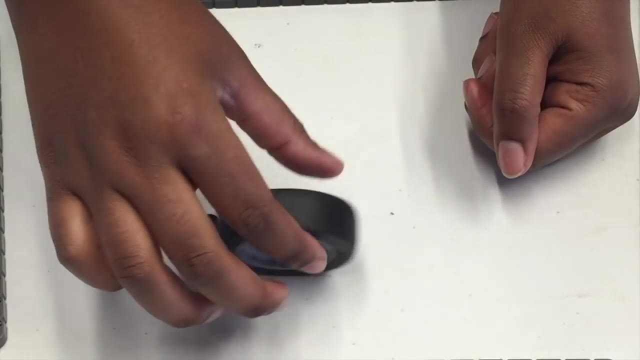 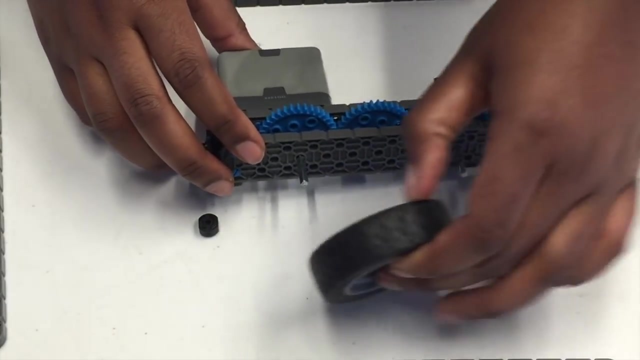 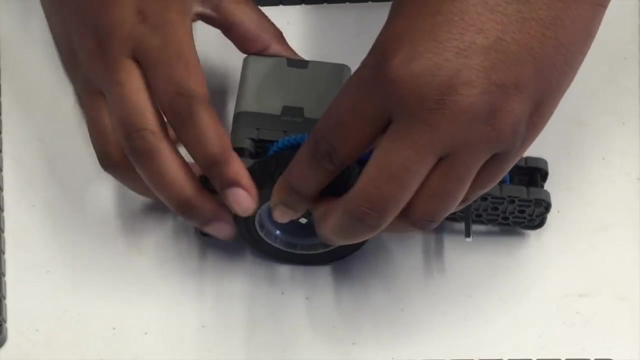 Just push that back until it's a nice fit. and now we have a wheel. Now grab your gearbox and your tire and place it on the wheel hub On top of our metal shaft. push that all the way back until I'll be and secure it with. 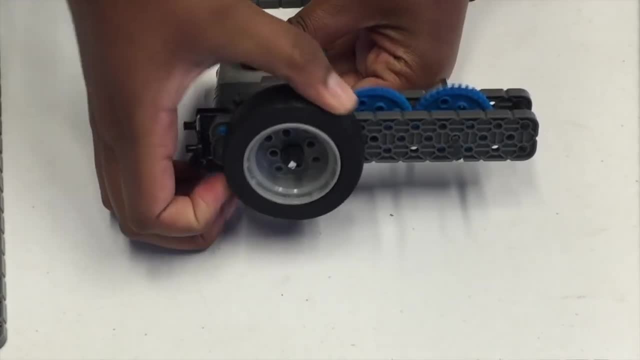 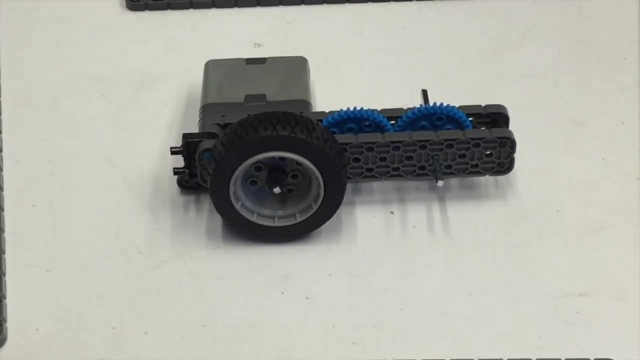 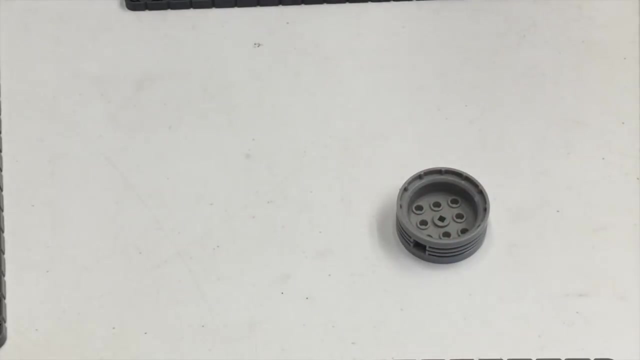 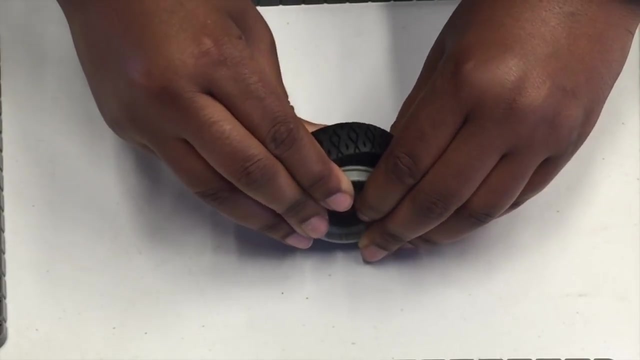 the shaft collar. Now, let's put that to the side. Let's grab our second wheel hub and our second tire. There we go. We're going to do the same thing we did to the first one: making sure the hollow part. 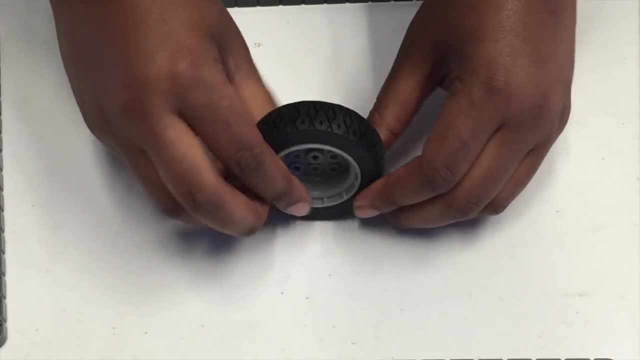 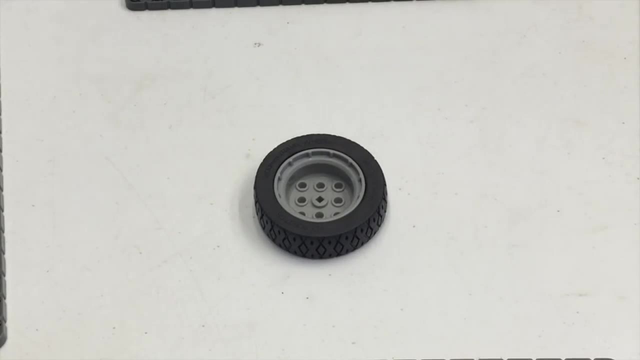 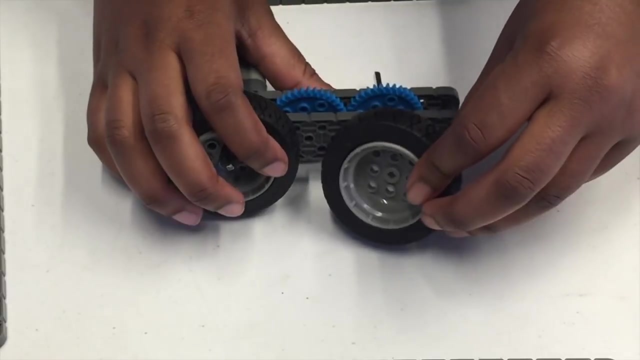 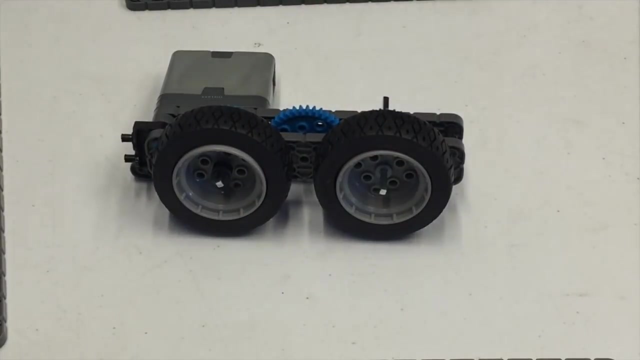 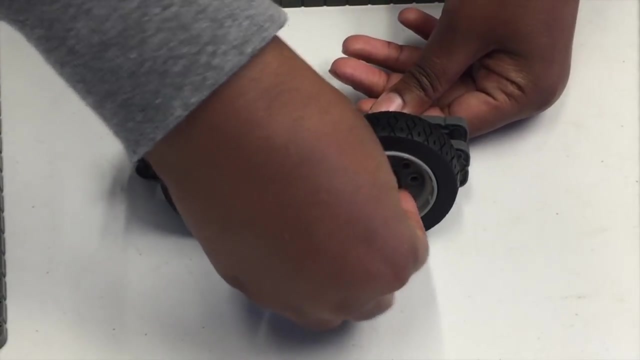 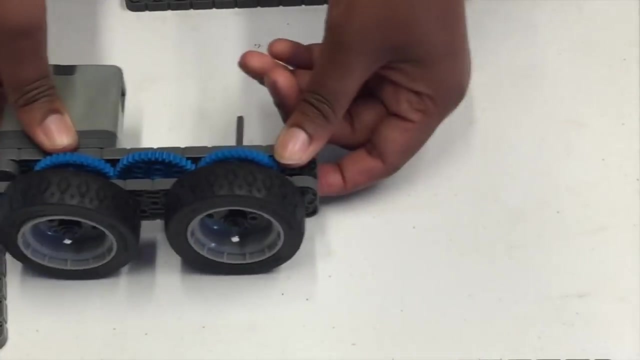 is facing out towards the letters, and push it back into the tire. Now grab out your gearbox and place your tire on your second open shaft and push it all the way back until it touches the beam. There we go. Now grab your shaft collar and put that right on top. 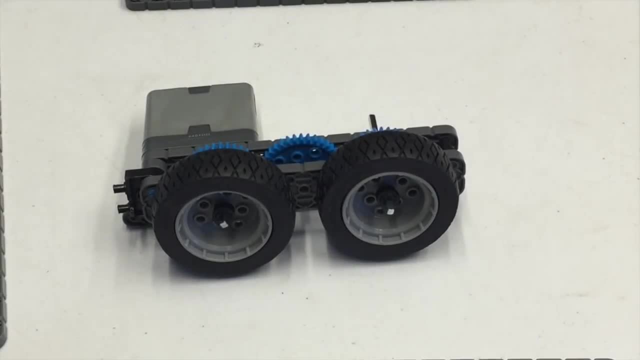 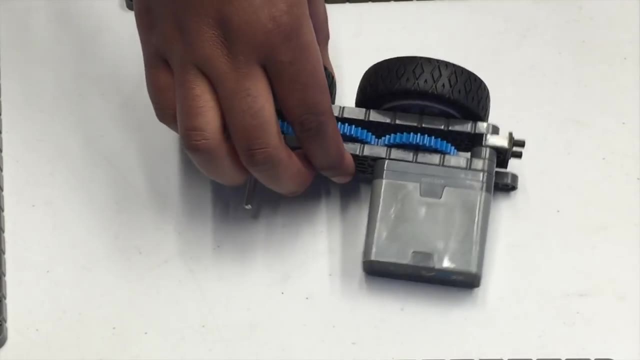 Now I'm just going to adjust the hub on top of the tire because it came off a little bit. Now, if you look at both angles, you should see the six-inch metal shaft sticking up the upper edge of the hub. Now, if you look here, you can see that the metal is sticking up the upper edge of the 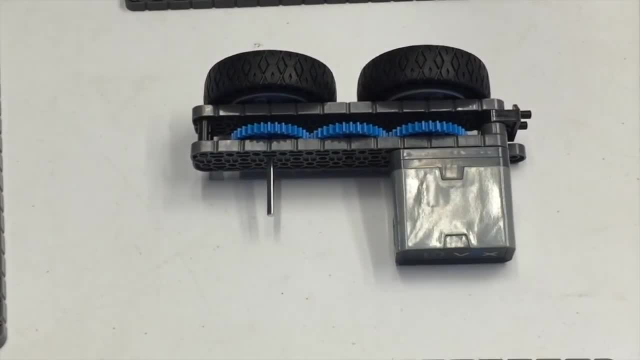 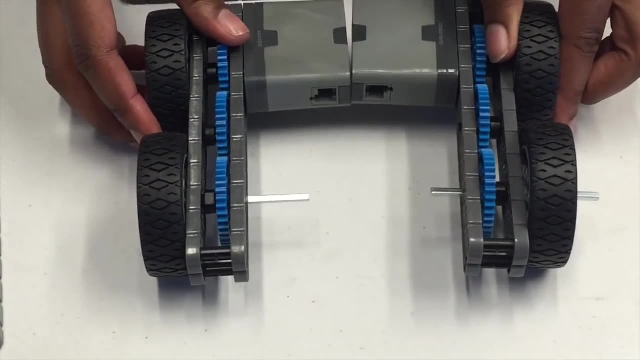 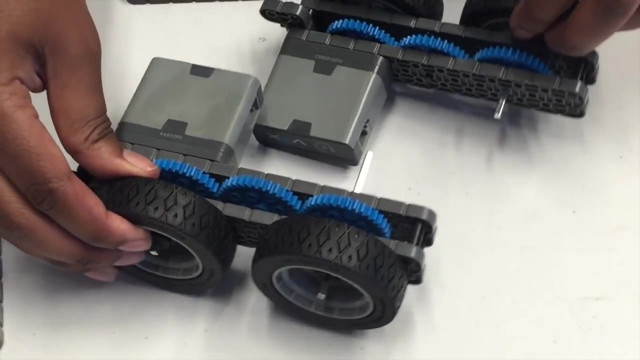 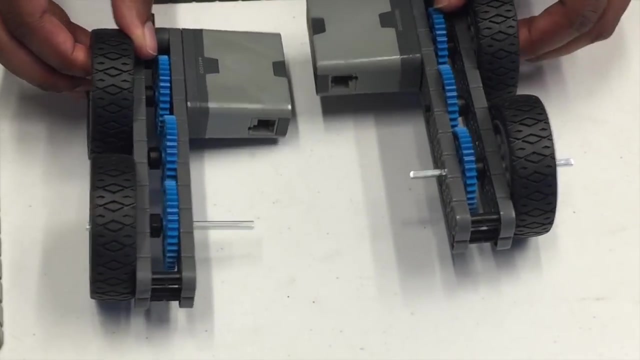 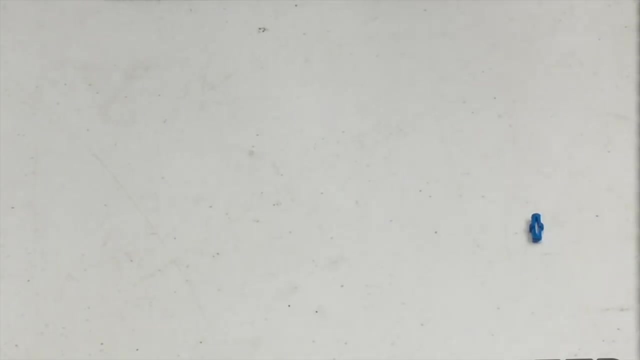 hub out on the opposite side. that is perfectly okay. you can leave that there. now, partner a and partner b: you can place both of your gearboxes next to each other and just double check that they are both identical. on to step seven. from this point forward, partner a and b will work together as a group. to finish, 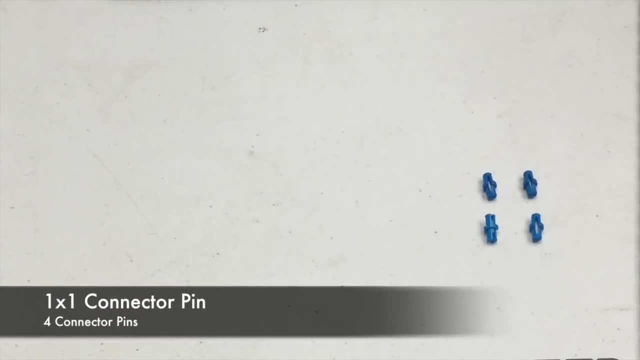 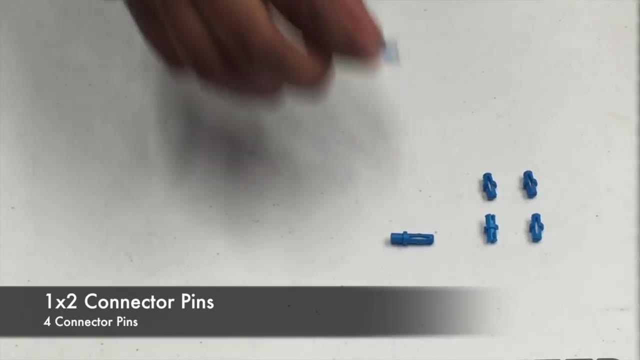 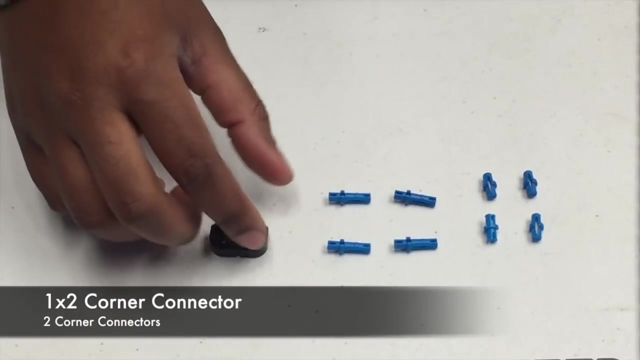 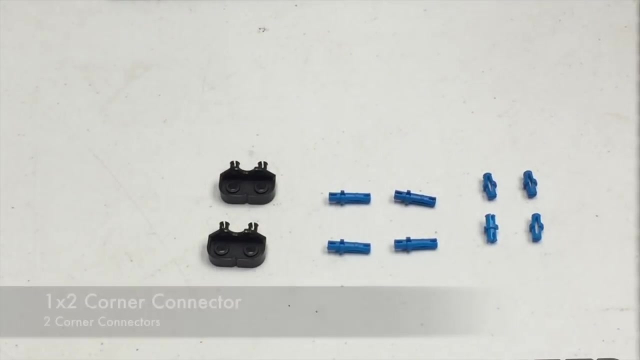 building their drive base. partner a can grab four one by one pin connectors, while partner b grabs four one by two pin connectors. you'll also need two one by two corner connectors and two three by five right ankle beams. make sure you count those holes out, so that you have seven holes in total. 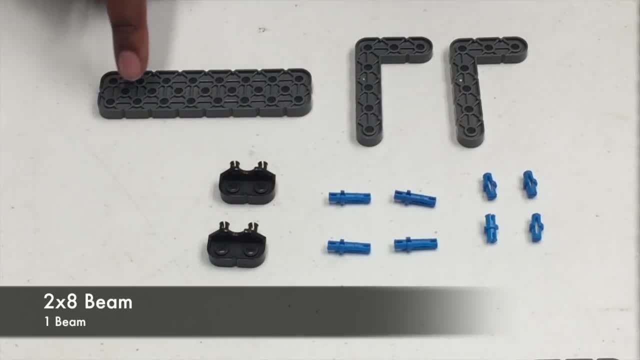 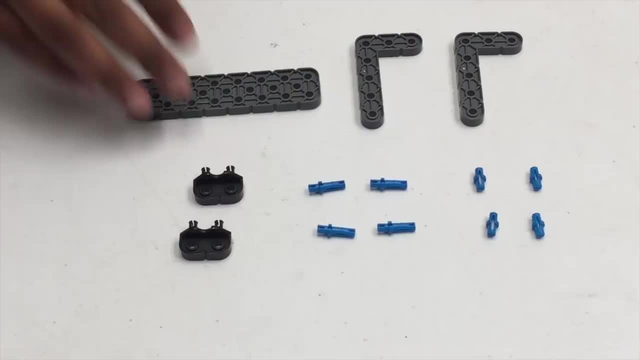 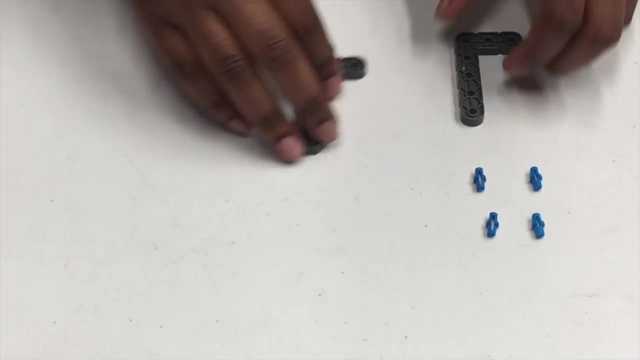 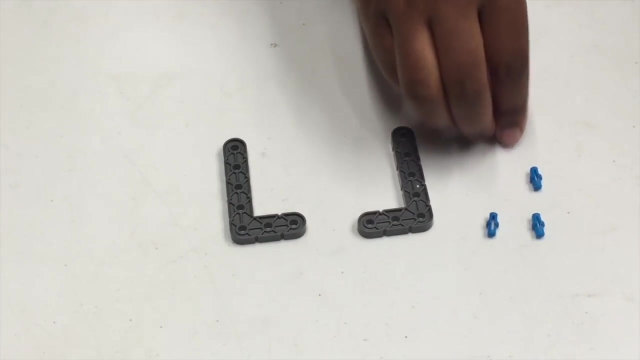 and lastly, you'll need one, two by eight and partner b. again, i'm counting the holes out. so there's eight across and two down. now partner a and partner b will each grab one three by five right angle bar and two connector pins and make sure they're both facing each other the way i have it here on the screen. 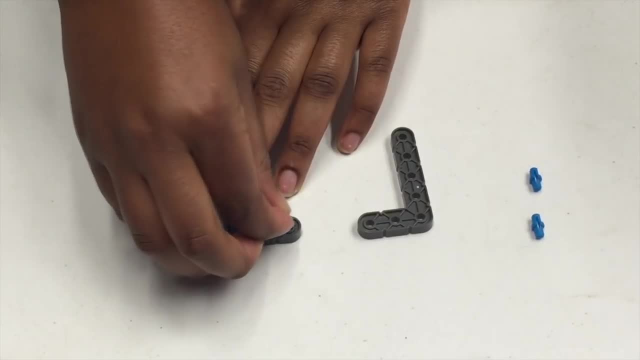 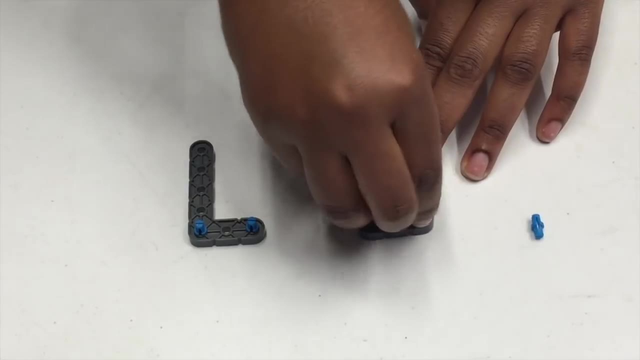 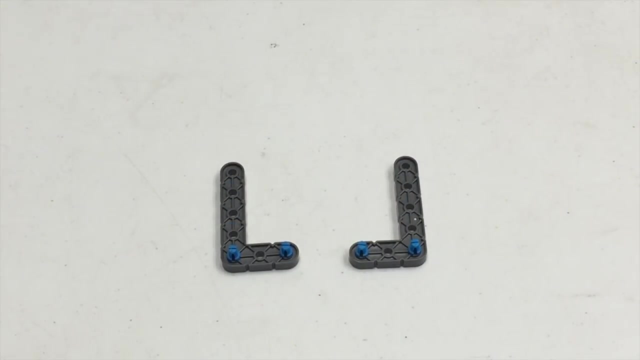 the first connector pin goes in the third hole and the second connector pin goes in the first hole. and then partner b- you'll do the same thing to yours- put one in the third hole and one in the first hole. now both partners put both of your three by five beams next to each. 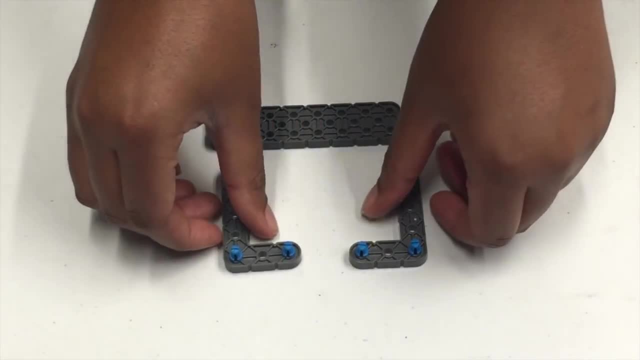 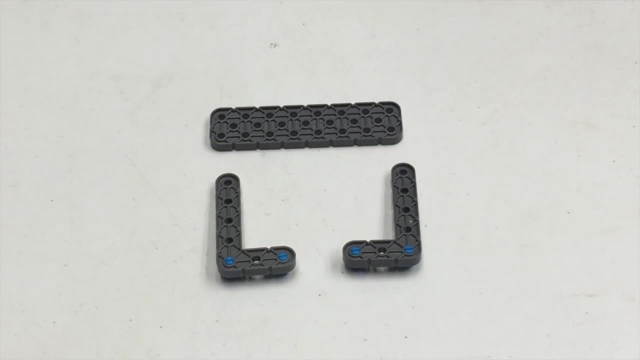 other to make sure that they are identical. now grab your two by eight beam and turn your three by five right angle beams upside down. Partner A: you grab two of the one by two connector pins, and partner B: you do the same thing. So first we're going to let partner A 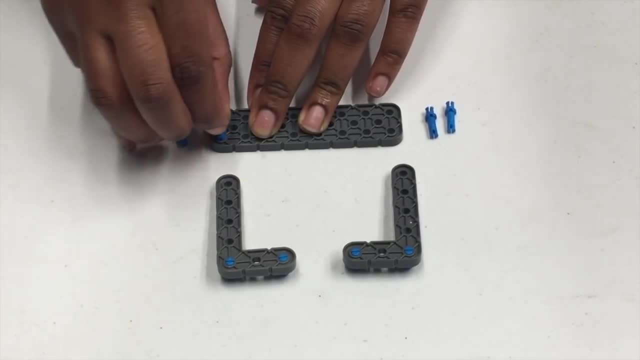 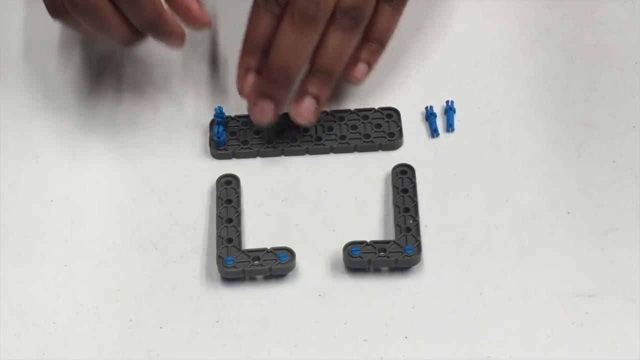 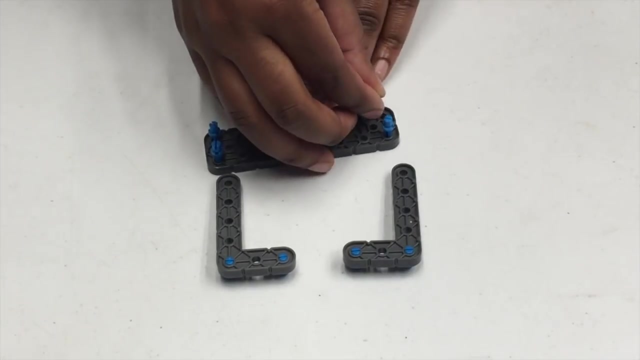 grab one of the one by two connector pins and place the long end down in the first hole into the two by eight beam and do the same thing with the second pin- Now partner B. you'll follow up with partner A by placing both of your connector pins down into the two by eight beam. 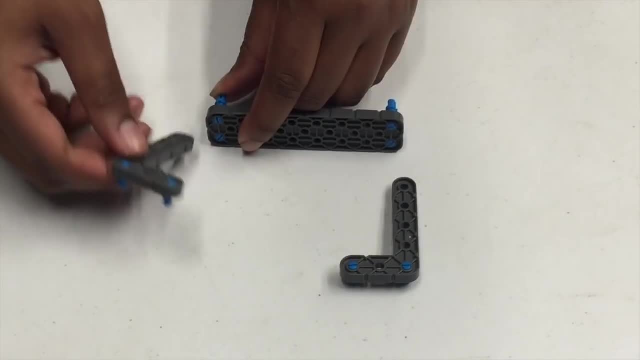 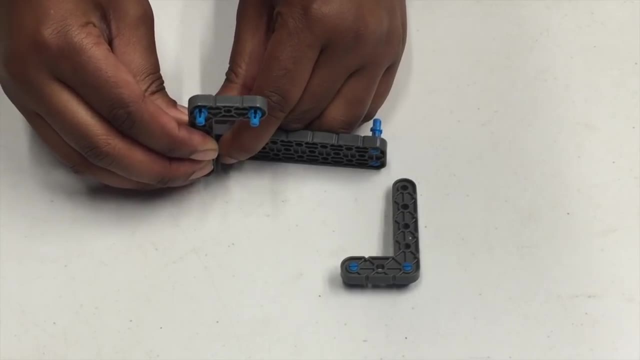 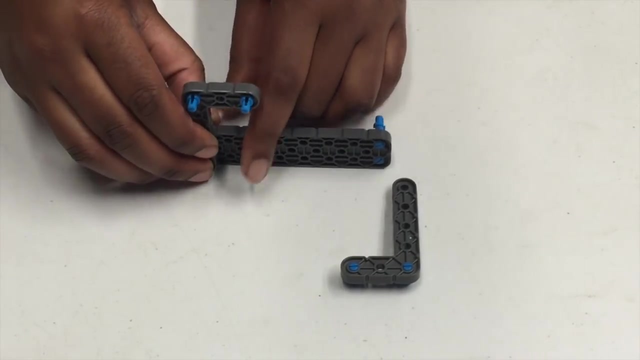 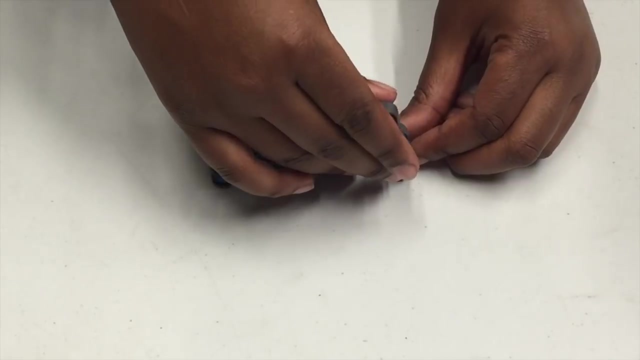 Now, partner A, grab your three by five right angle beam and you want to place that directly against the two by eight beam and press your one by two connector pin all the way through until it is holding the right angle beam in place. Once partner A is finished, partner B, you will grab your right angle beam. 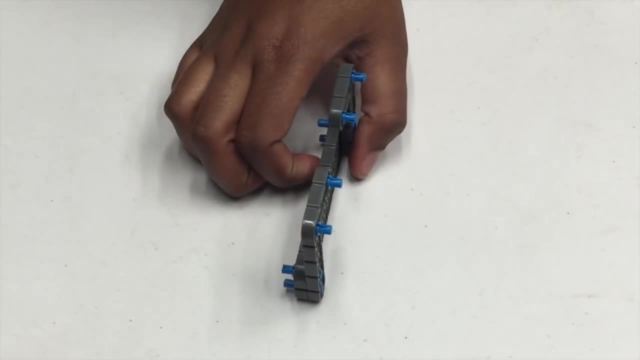 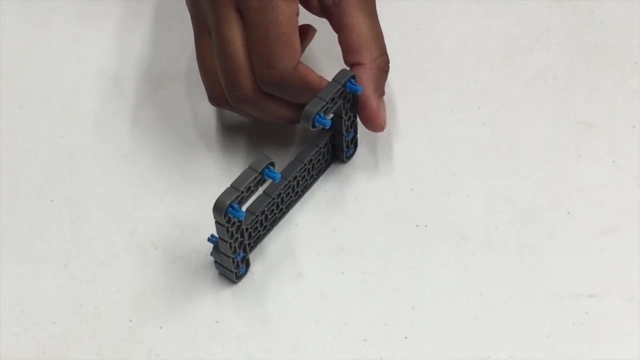 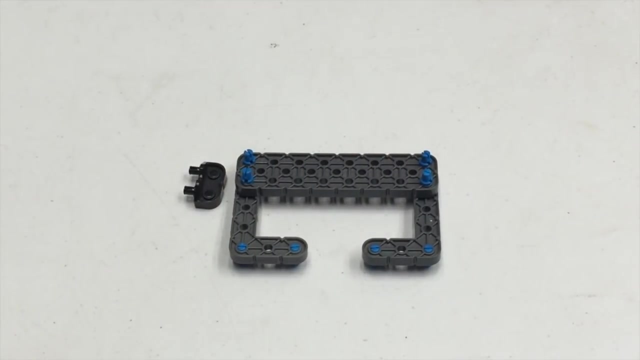 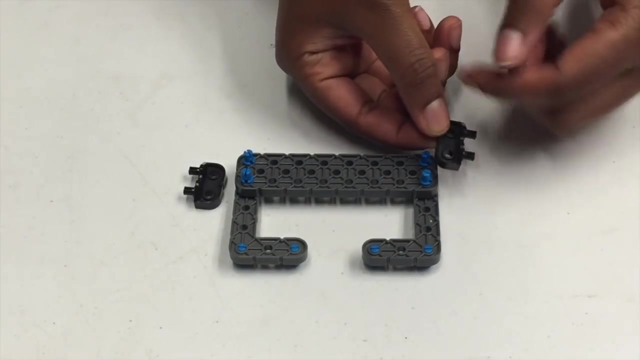 and do the same thing to the other side. Now you should have a two by eight beam connected to a three by five right angle beam. Now, partner A, grab your one by two corner connector and partner B, do the same thing and you want the pins to be facing out away from the structure. 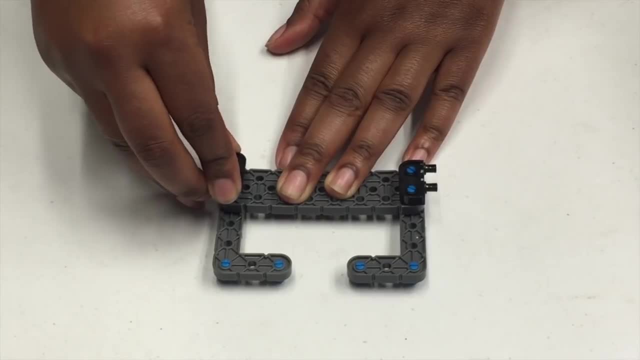 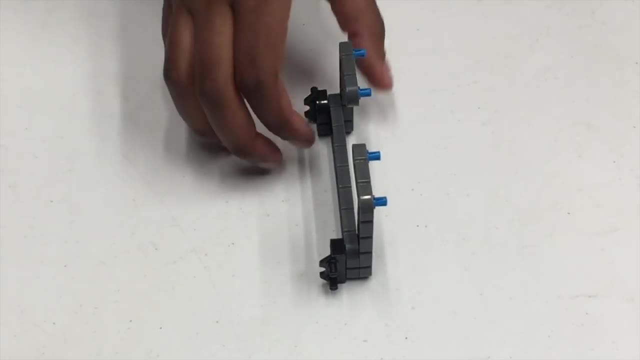 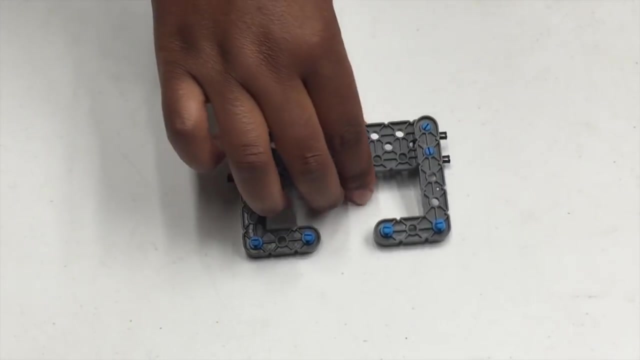 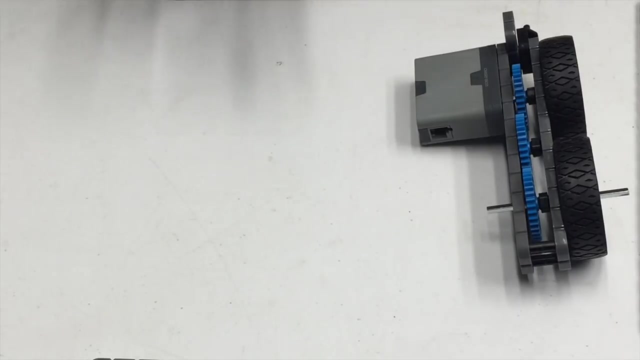 and you're going to snap both of those on to the structure you already made. So now, when you stand it up, only thing you should see are four connector pins sticking out of the 3x5 right angle beam, Step 8,. partner A: you will need to grab your gearbox and partner B: you will do. 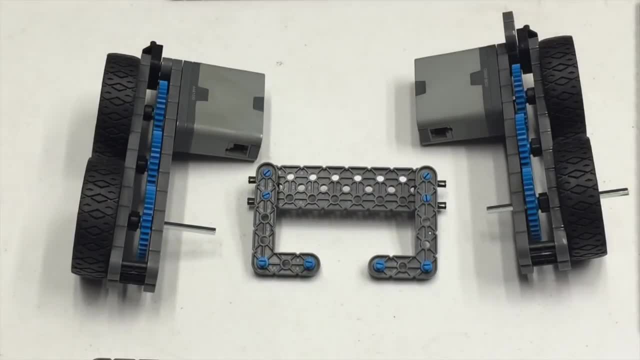 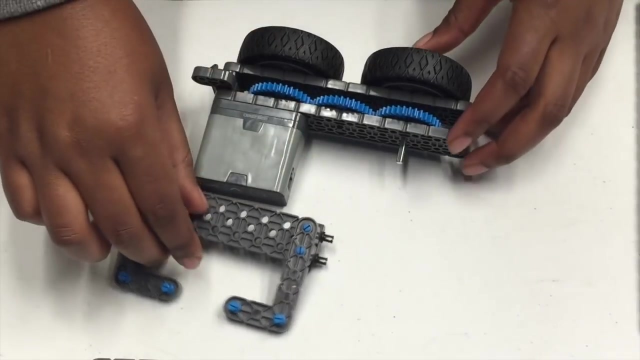 the same thing, and for this step you will also need the structure that you just created in step 7.. So first we're going to start with partner A, You're going to grab your gearbox and the structure that you just made and you're going to count out. 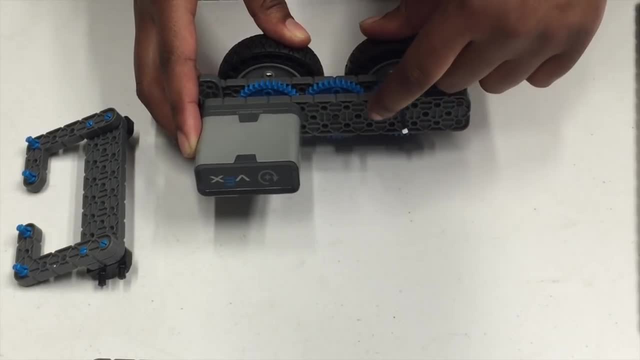 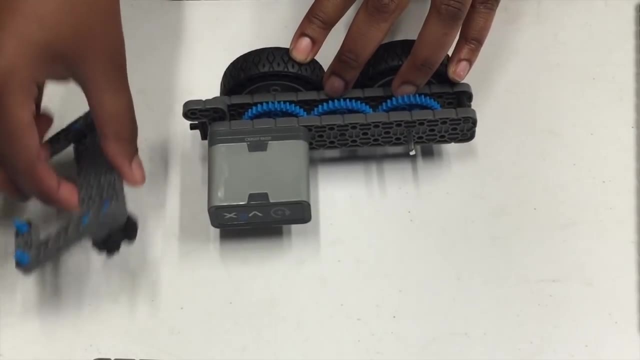 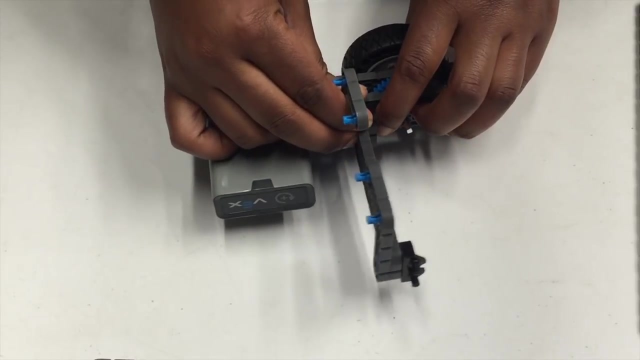 the two columns away from the shaft, 1, 2, and we're going to grab our structure, making sure that the blue pins are facing towards the motor and the black pins are facing towards the wheel, and we're going to snap that right in place. 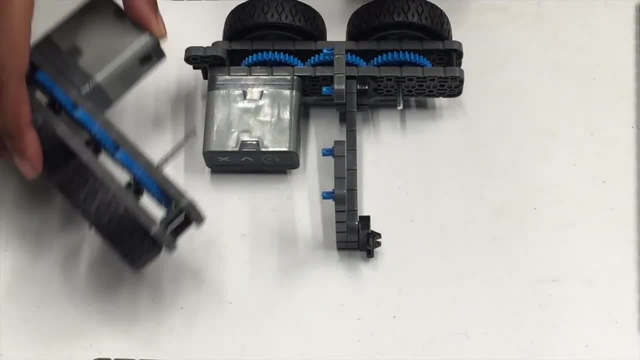 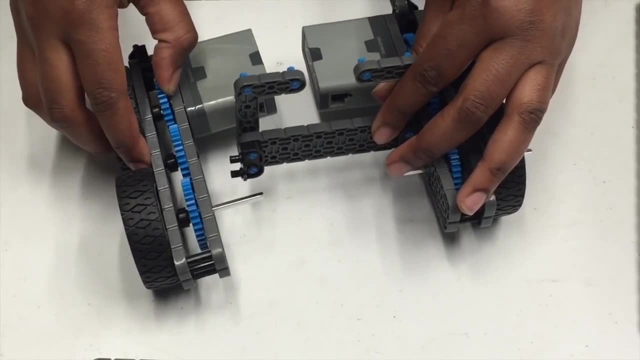 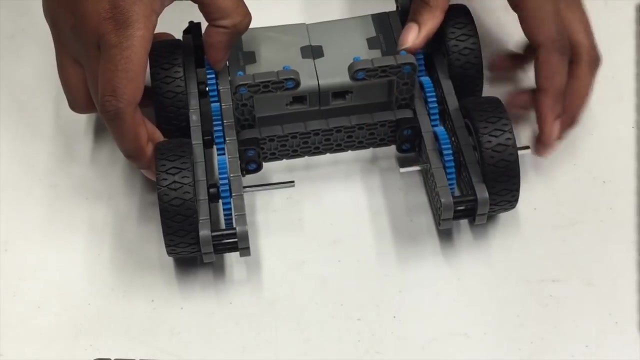 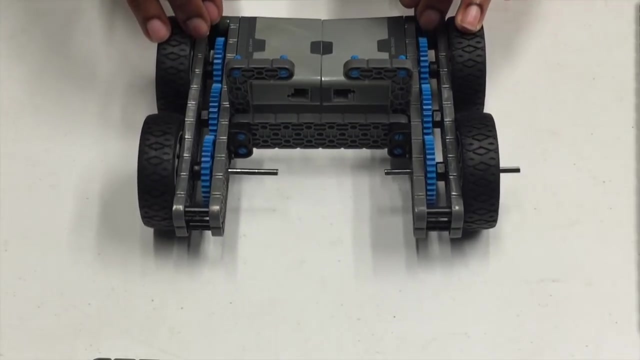 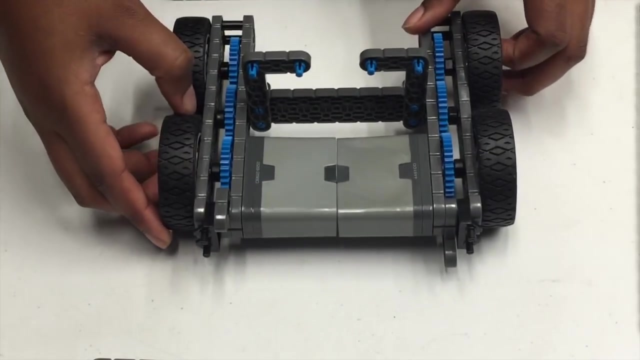 Again. notice the blue pins are facing towards the motor. Now, partner B, you're gonna grab your gearbox and do the same thing partner A did, and count out two columns from the metal shaft and snap the corner connector onto your gearbox. so now a robot is starting to look more like an actual drive base. Again, notice that it's not against the instrument. We want to make sure that we're sleeping in the center some overall looking of our architecture project. so notice about pinpoint freedom and that, and to the tip of the thread, we're putting our electric cable onto the drive. 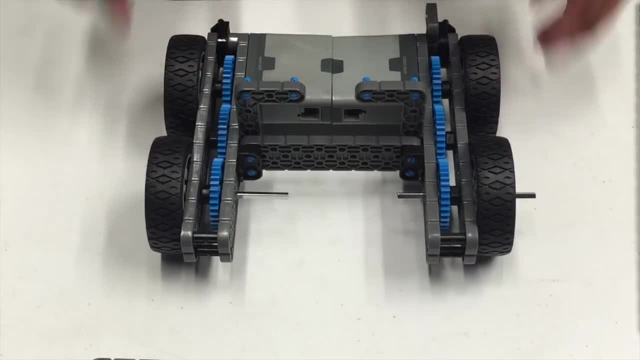 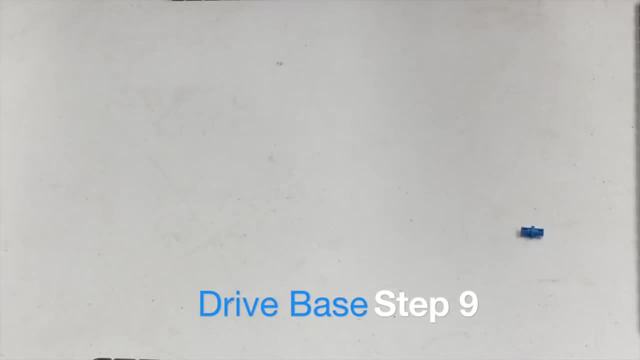 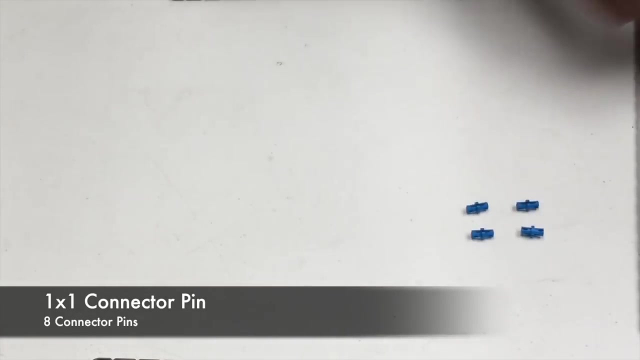 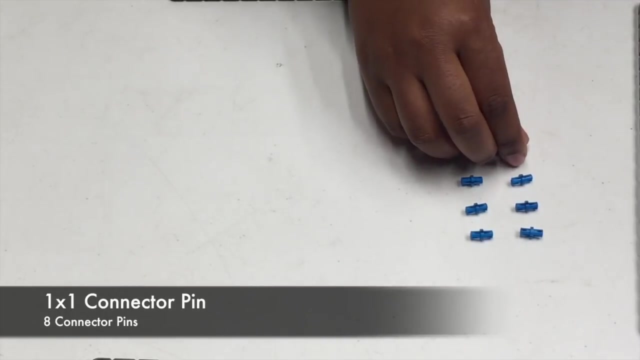 that all four of the connector pins should be facing towards the back of the drive base On to step nine. Again, for this step, partner A and B will work together, so you will only need eight, one by one, connector pins that both partner A and B will count out and share together. 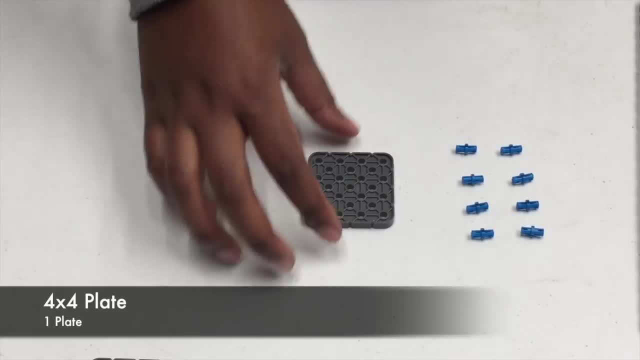 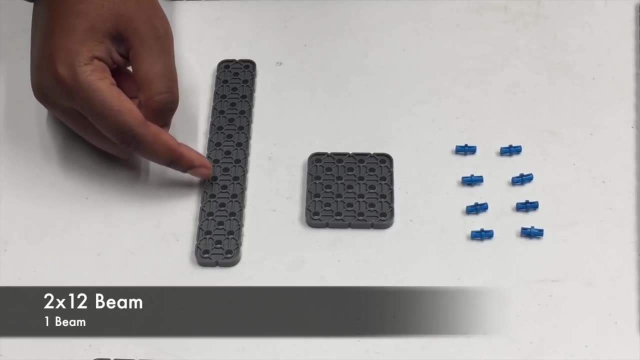 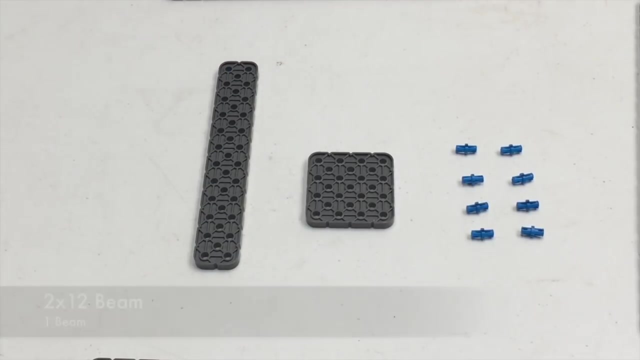 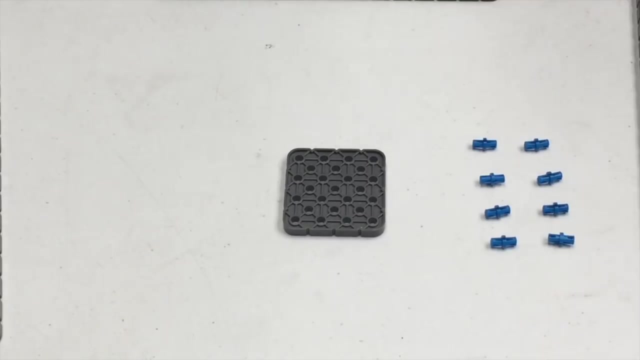 You'll need one four-by-four plate and one two-by-twelve beam. You see me counting out the holes, making sure again that I have the correct beam. There should be two across and 12 down. Now sit that two by twelve beam to the side and partner A you can grab. 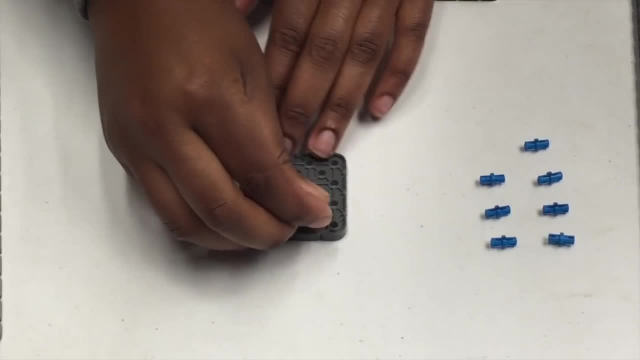 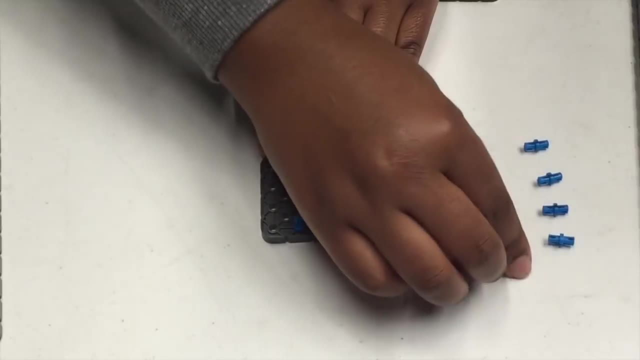 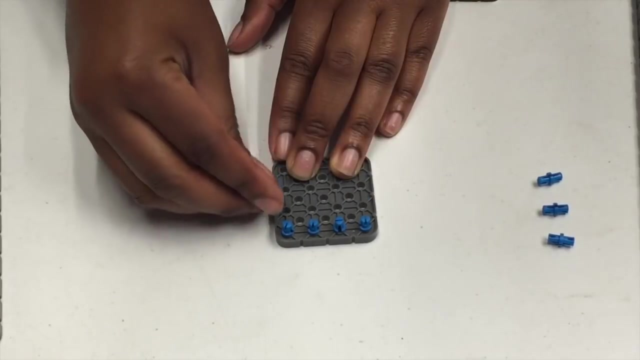 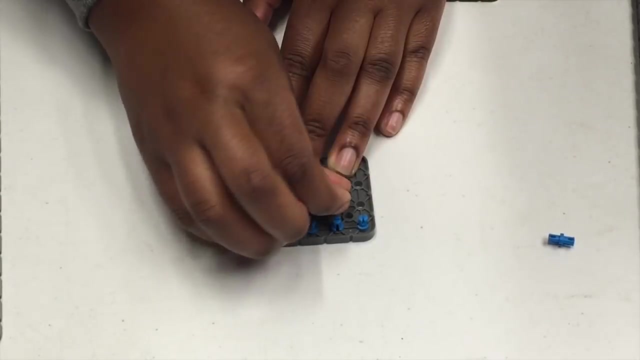 four by four, four of the 1x1 connector pins and place them in the bottom row of the 4x4 pleat. Partner B: get ready Now. once partner A is done, you will follow up by placing your four 1x1 connector pins in the second row of the 4x4 pleat. 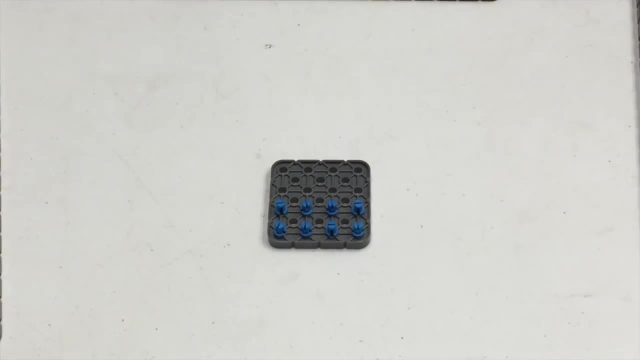 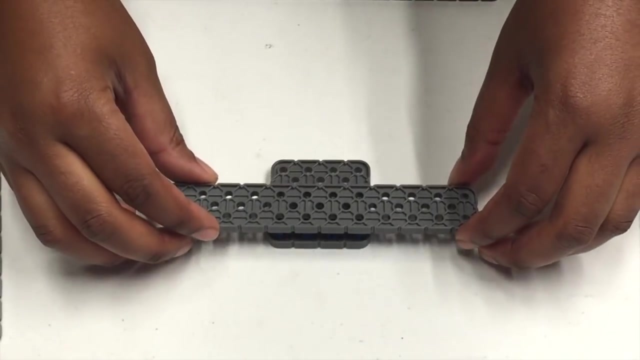 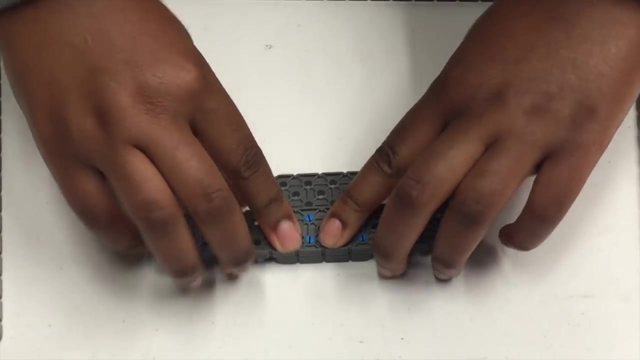 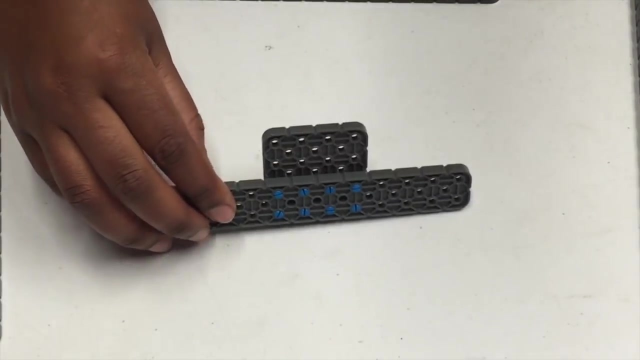 Now that that is completed, one of the partners can grab the 2x12 beam and place it directly on top of the 4x4 pleat. You want to make sure it's centered, so there should be four open holes on each end of the 2x12 beam. 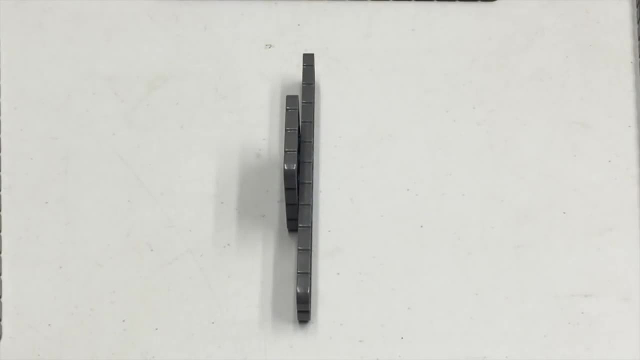 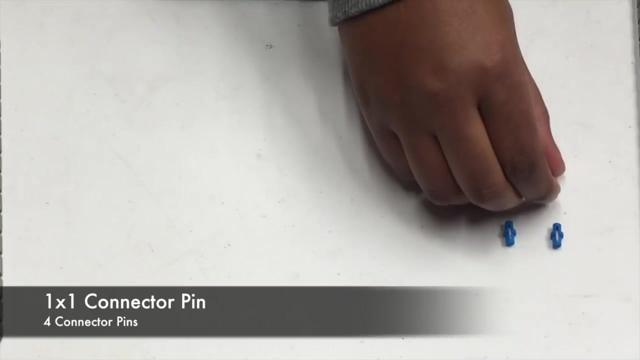 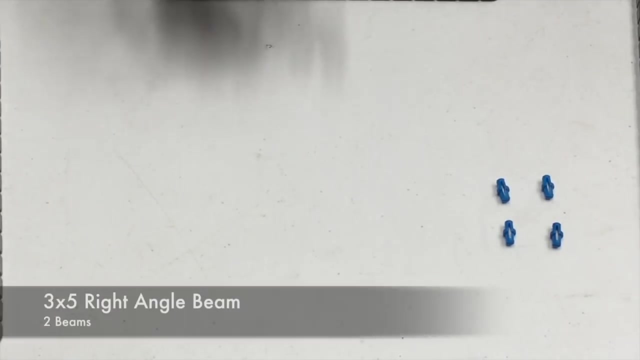 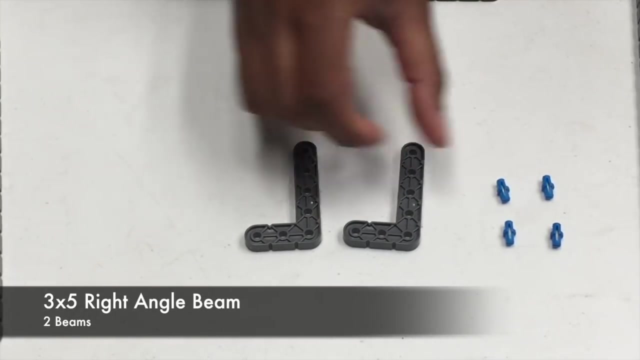 Make sure that none of the connector pins are sticking out past the beam Time for step 10.. Partner A and B: you will need to together get four 1x1 pin connectors, two 3x5 right angle beams and a 3x5 right angle beam. 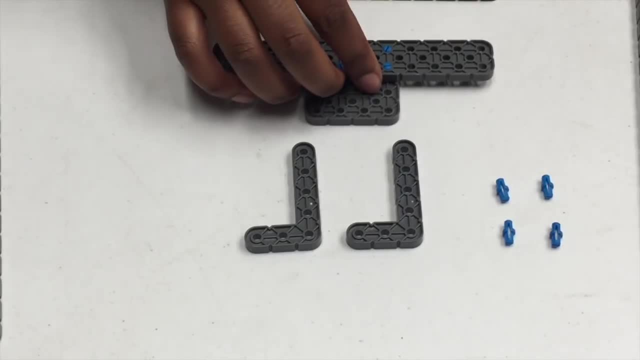 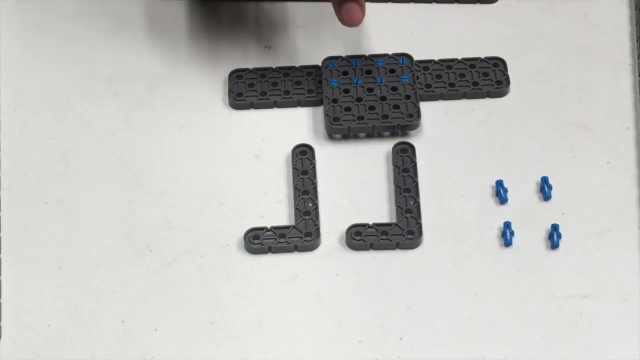 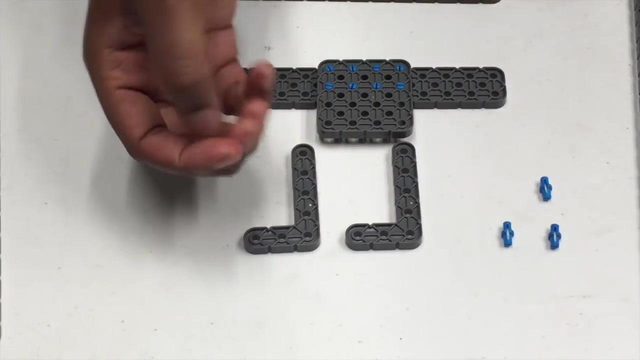 I'm counting them out, making sure that there are seven holes there and you can bring in the structure that you just created in the last step. Now turn the beam over so that the 2x12 beam is against the table and the plate is sticking up in. 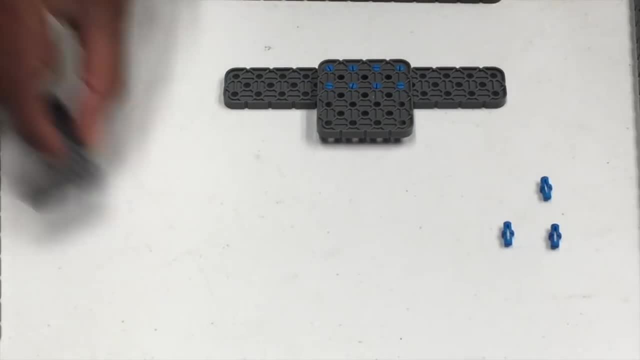 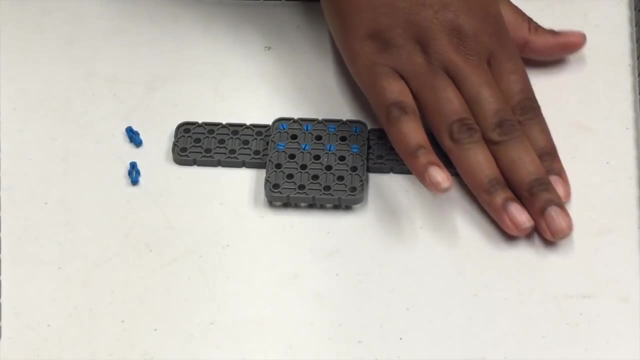 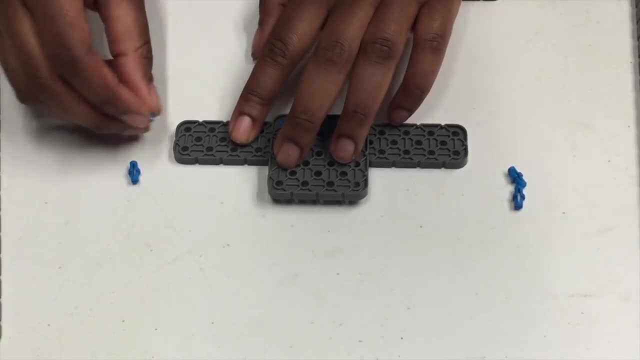 the air. You are going to share the pieces with each other, so partner A should have two 1x1 connector pins and partner B should have two 1x1 connector pins. Now let's count to the third hole and we're going to put one 1x1 connector pin in the top row and 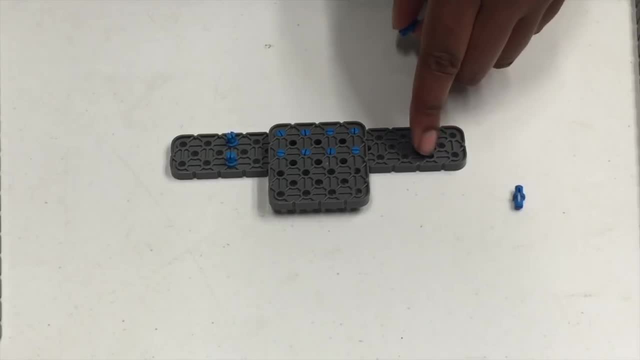 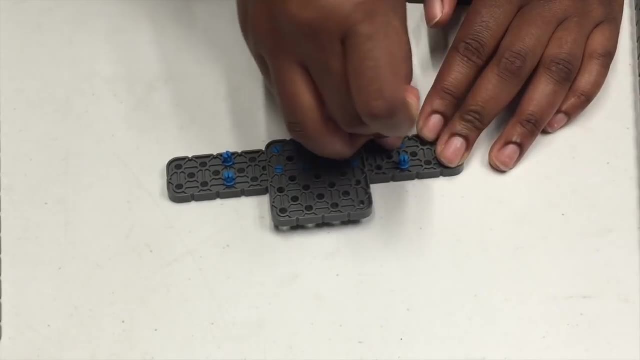 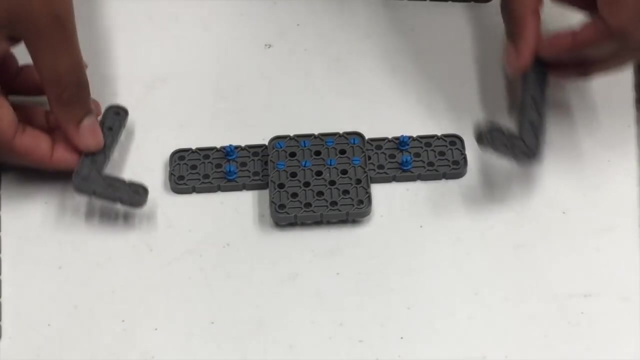 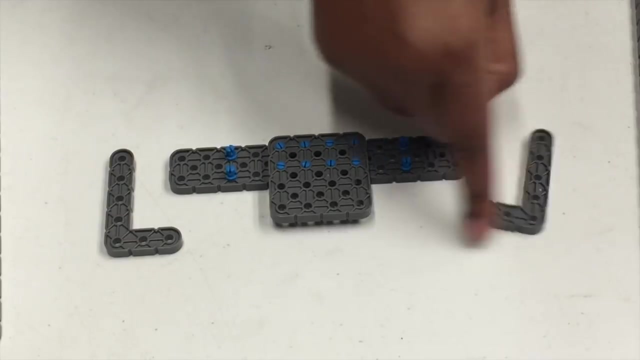 one in the bottom row. Partner B: you're going to do the same thing. count to the third hole and put one 1x1 connector pin in the top and one 1x1 connector pin in the bottom row. Now each partner grab one 3x5 right angle beam and make sure that they're both facing towards. 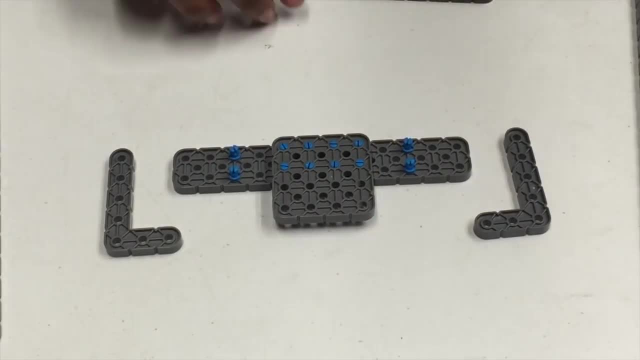 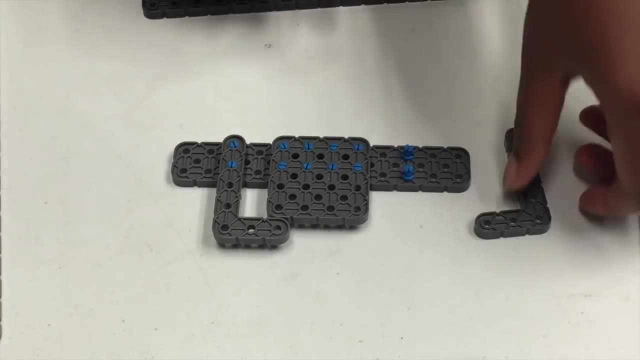 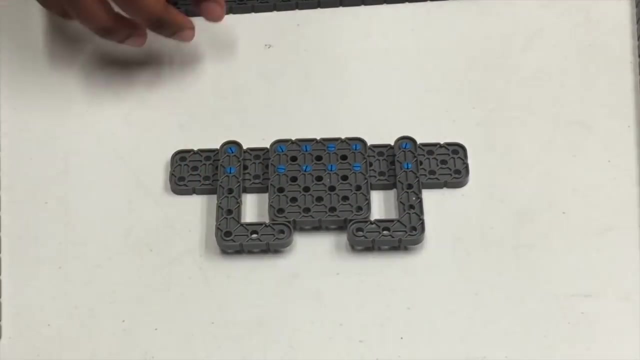 each other. and then you're going to place that 3x5 right angle beam on top of your structure so that again, both of the beams are pointed towards each other. and then you're going to put one 1x1 connector pin in the top and one 1x1 connector pin in the bottom. 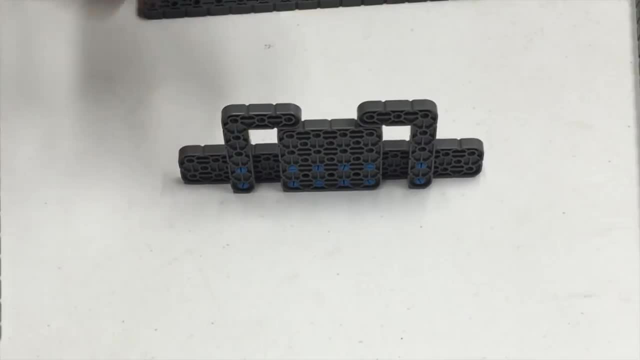 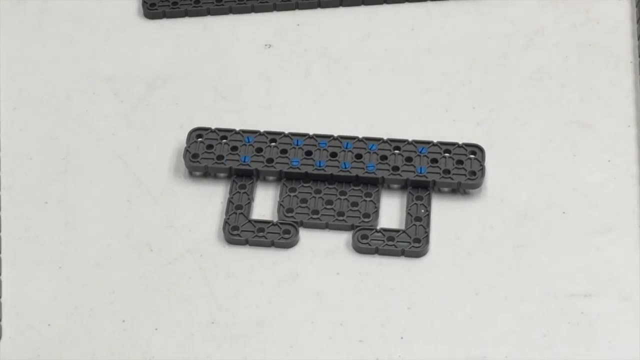 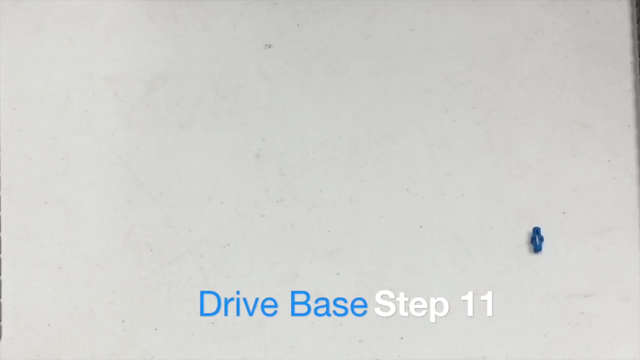 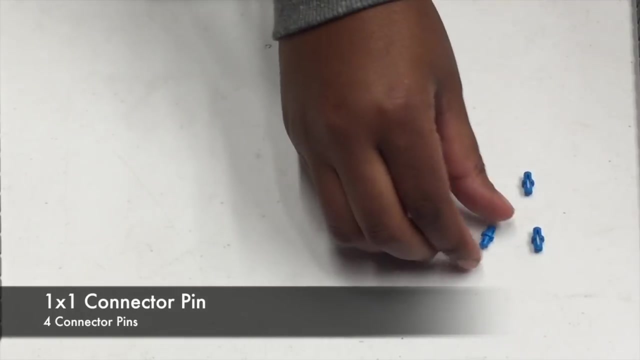 row. Now, when you lift up your beam, you should have again no connector pin sticking out of the structure. Step 11, partner A and B: you are going to work together to get four 1x1 connector pins and two 1x6 connector pins. 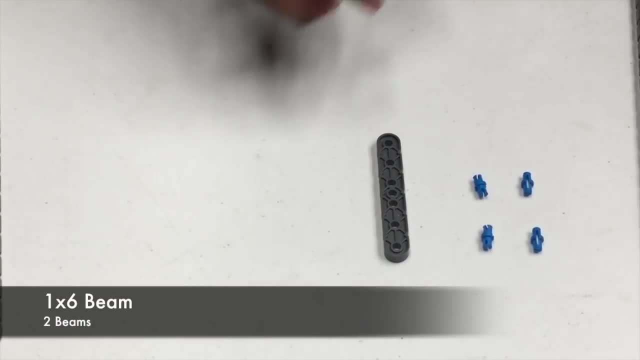 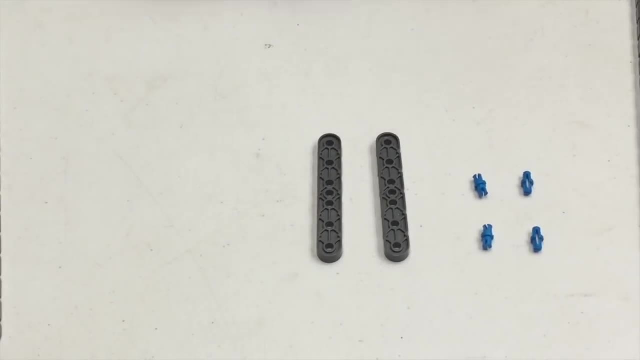 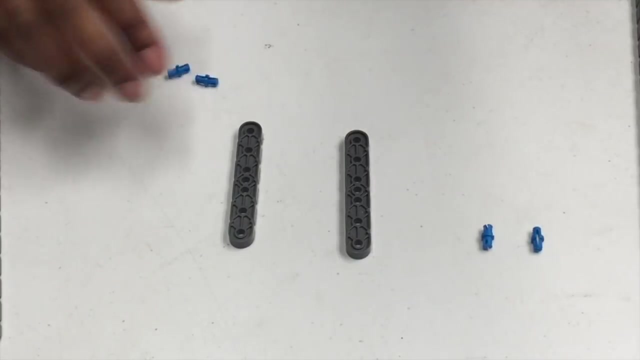 And two 1x6 connector pins This beam. you'll need to count out to make sure that you have seven holes on the beam. Now it's time to share the pieces. Partner A: you will grab two of the 1x1 connector pins and. 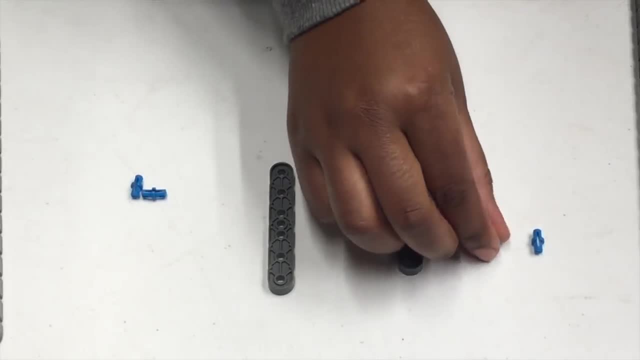 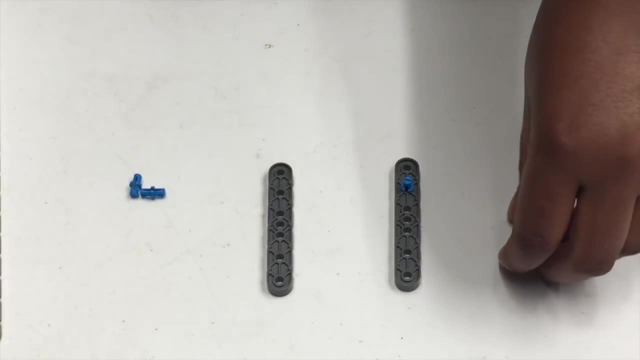 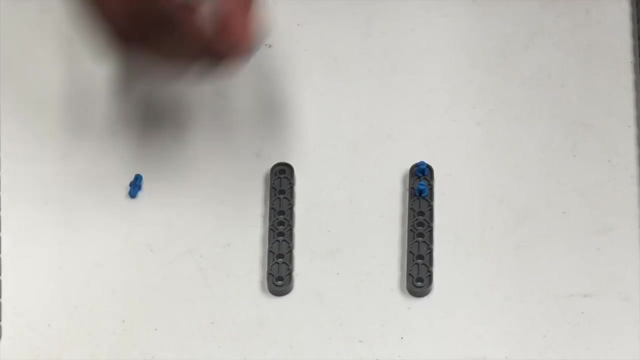 one of the 1x6 connector pins And partner B. you will do the same thing. The first 1x1 connector pin will go in the second hole and the second will go in the bottom hole. Both partners beams should look identical to each other. 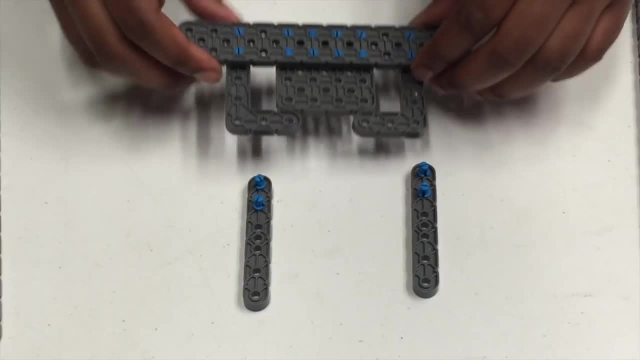 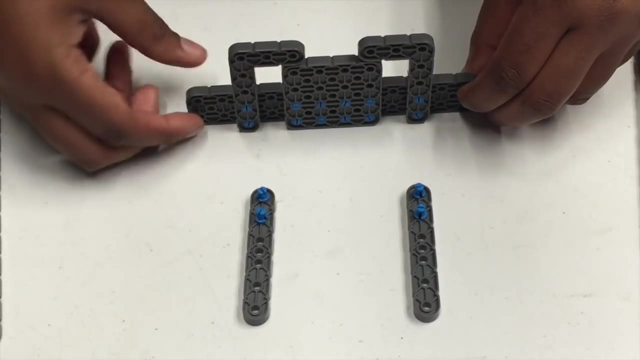 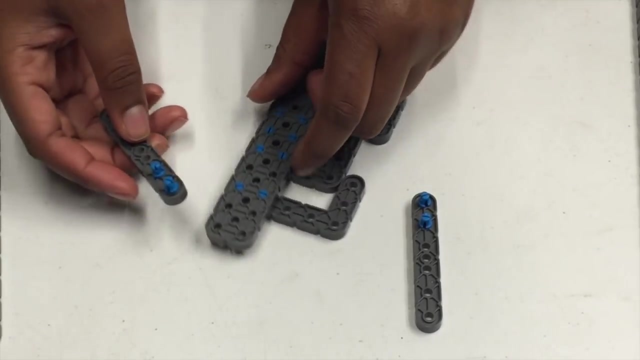 Now grab your structure that you made in the previous step and flip it over so that the plate and the angle are sitting against the table, Each partner. grab your 1x6 beam and place the two connector pins in the bottom two holes of the 3x5 right angle beam. Now you'll have to make sure that the 3x5 right angle beam is in the center of the 2x5 angle beam. So you're going to do that. you're going to do that. You're going to do that. 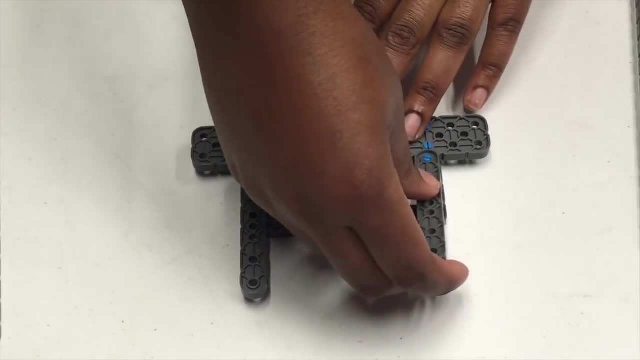 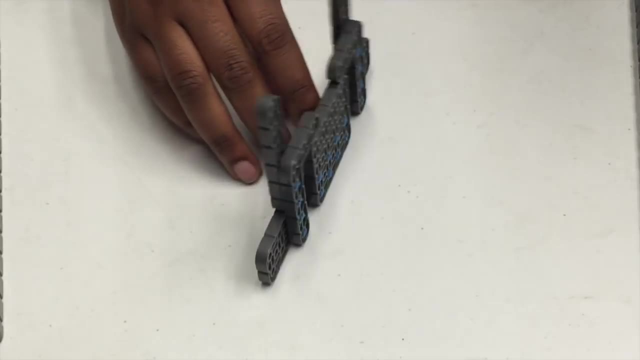 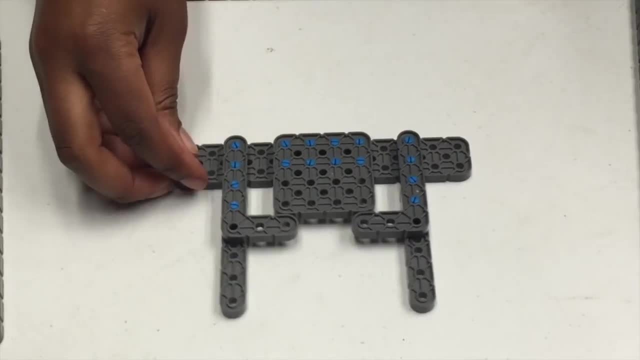 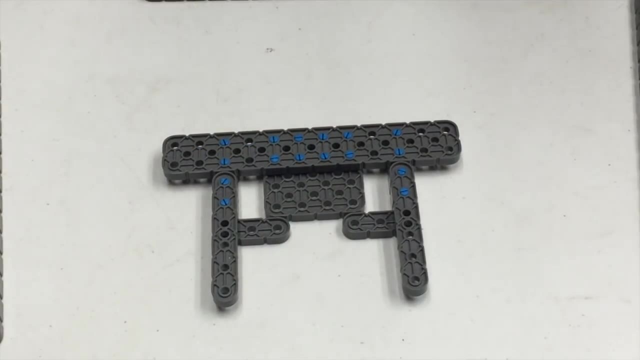 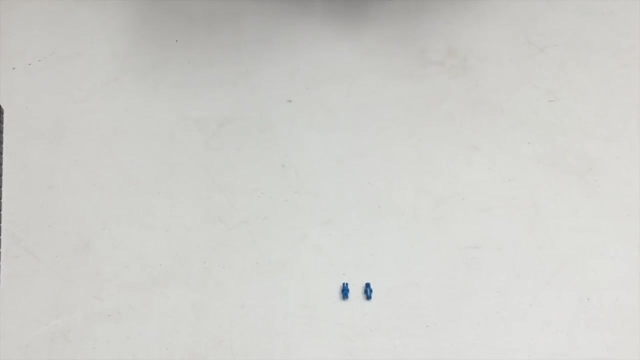 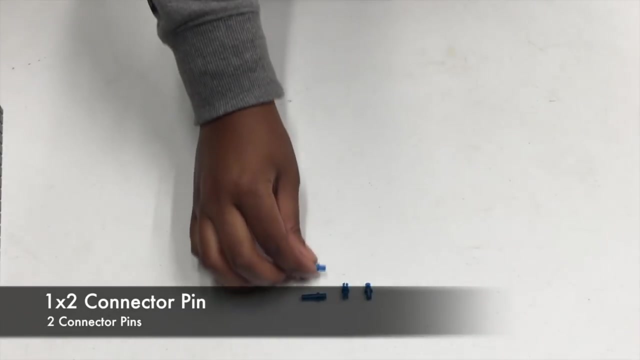 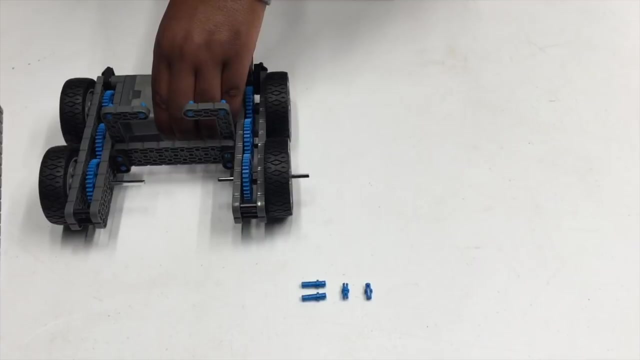 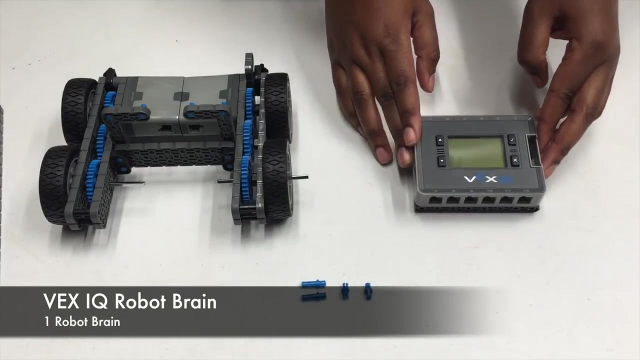 pins sticking out past the structure- Step 12,. one of the partners will need to get two 1x1 connector pins, while the other grabs two 1x2 connector pins. You will also need to get your cart that you already made and one VEX IQ robot brain You can place. 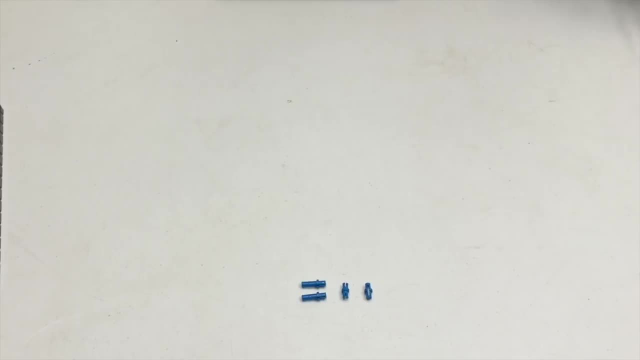 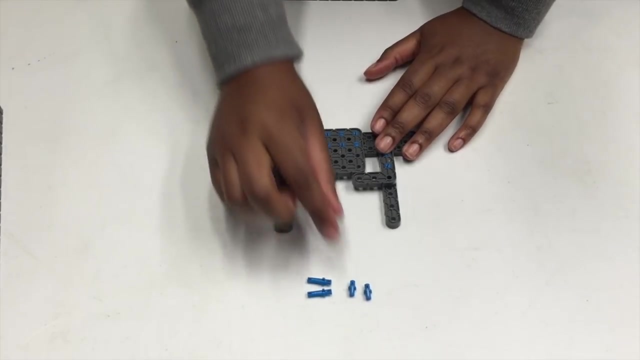 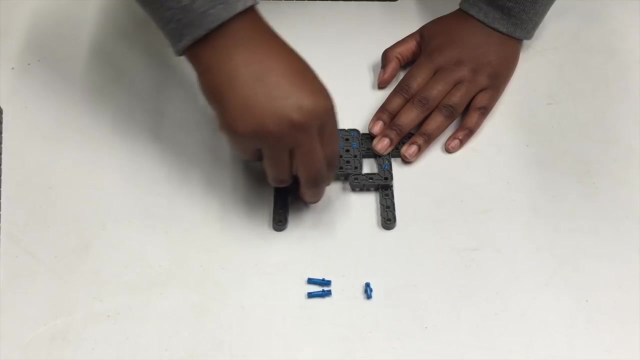 your cart to the side for now and bring in your structure that you just made in the previous step And you want to lay it down so that the 2x12 beam is against the table Now. one of the partners will first grab one connector pin and place it in the furthest. 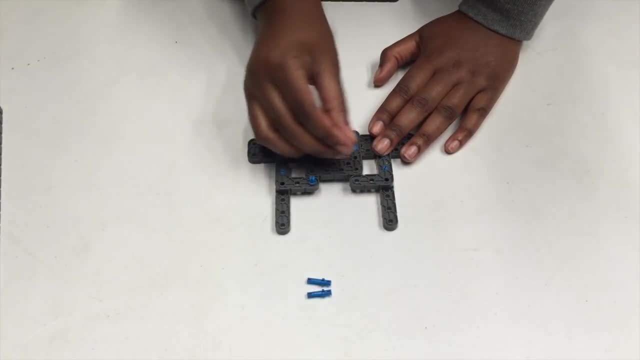 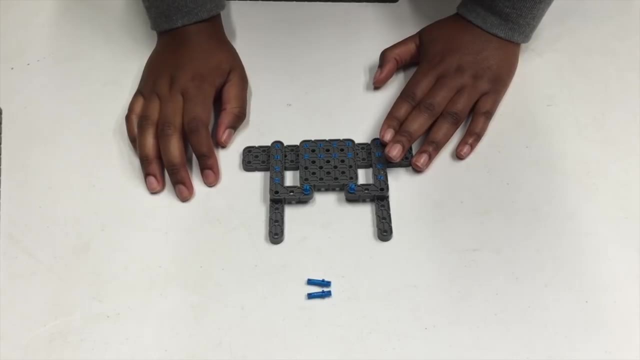 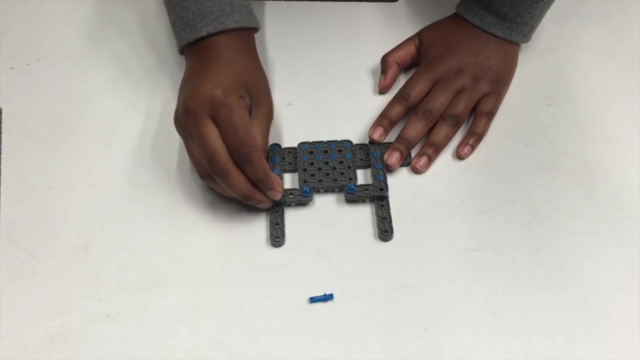 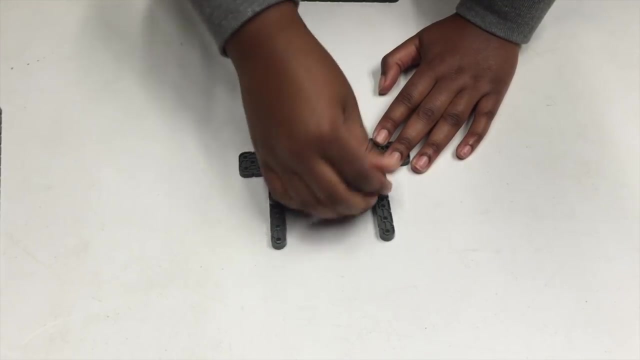 hole on the 3x5 right angle beam, While the second partner will place another 1x1 connector pin on the 3x5 beam on the other side. Now grab your 1x2 connector pin and place the long end of the 3x5 right angle beam so that it connects to the 1x6 beam, And do the same thing to the. 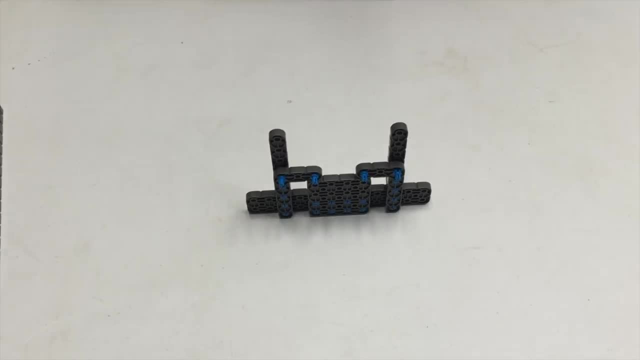 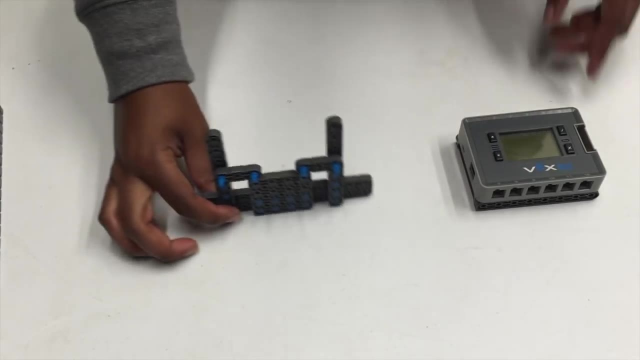 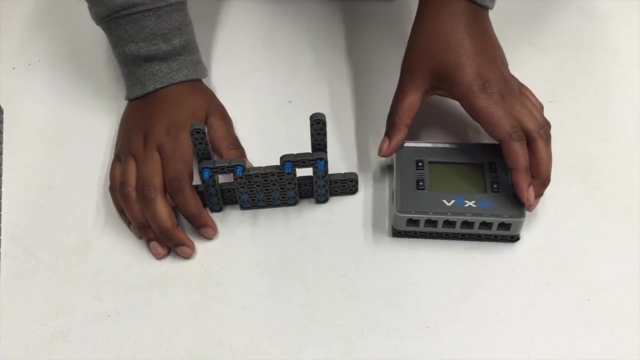 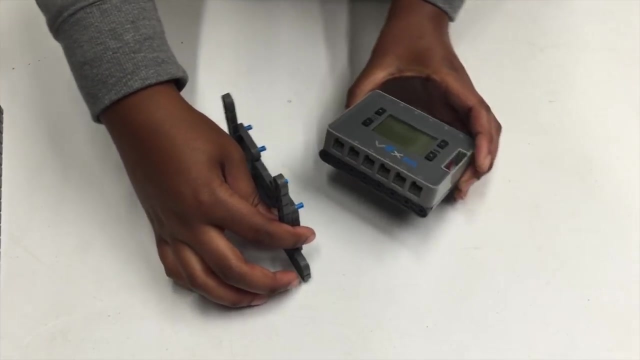 other side. You should now have four connector pins sticking out of one side of your structure. Now grab your VEX IQ robot brain and make sure that you have numbers 1-6 facing towards the structure. Now. you'll be able to see the VEX IQ robot brain in the frame right now And you'll notice. 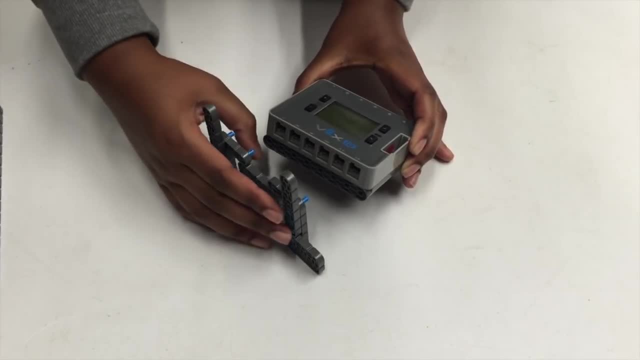 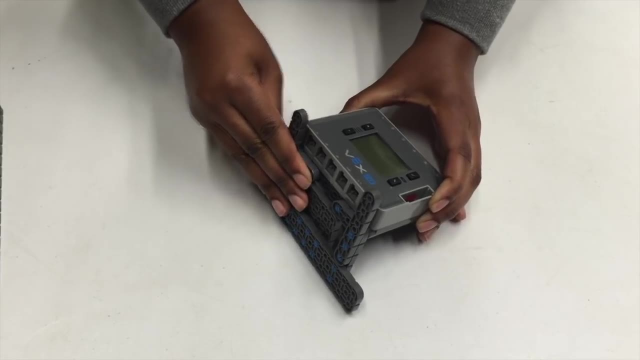 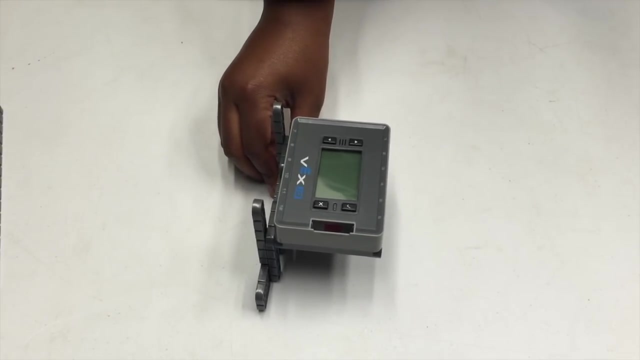 the beam on the bottom of the robot brain. You're going to line your structure up with the VEX IQ robot brain and snap it directly against it so that it's flat. You can see that the VEX IQ robot brain has a right angle beam on the bottom of the. 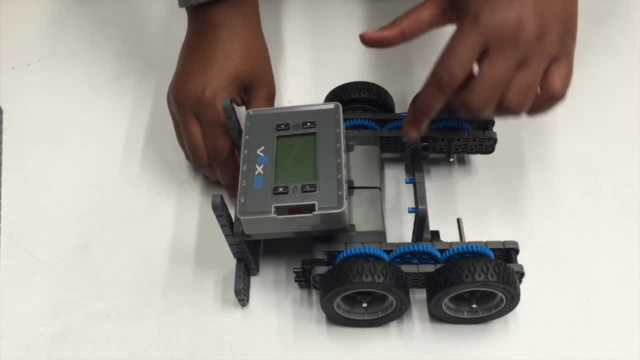 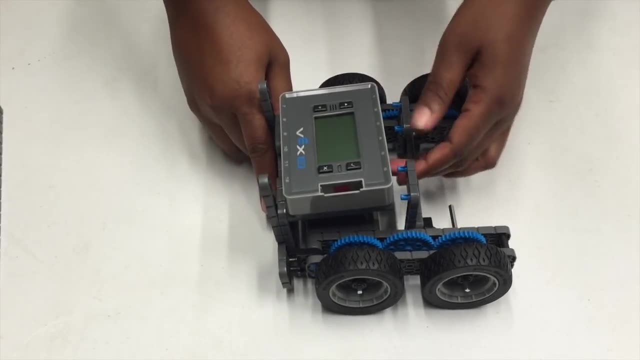 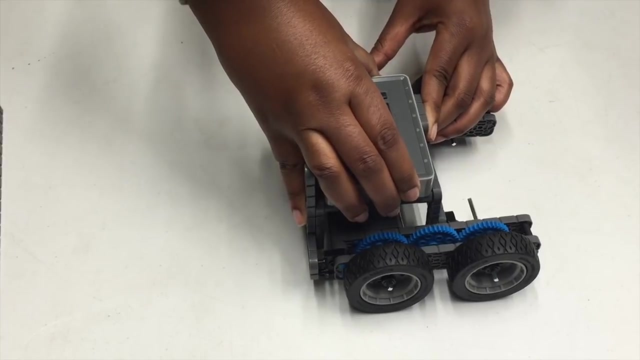 frame. Now grab your cart and line it up so that it's flat. The four connector pins are on the right angle, facing numbers 7 through 12, and you're going to snap those into place as well. Once you have all four of the 1 by 1 connector pins together, turn the drive. 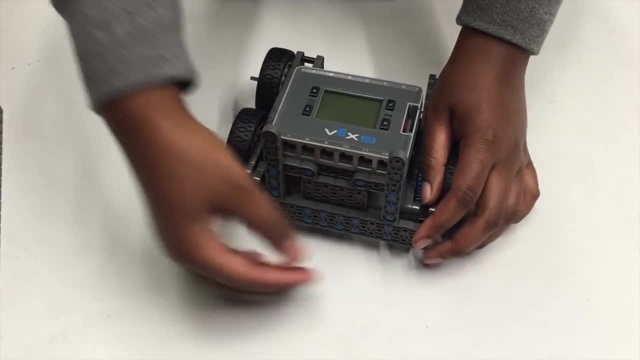 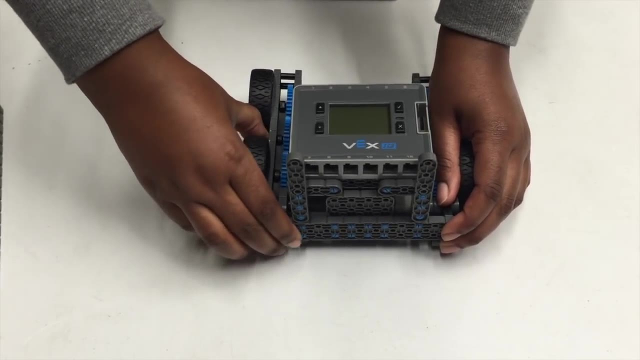 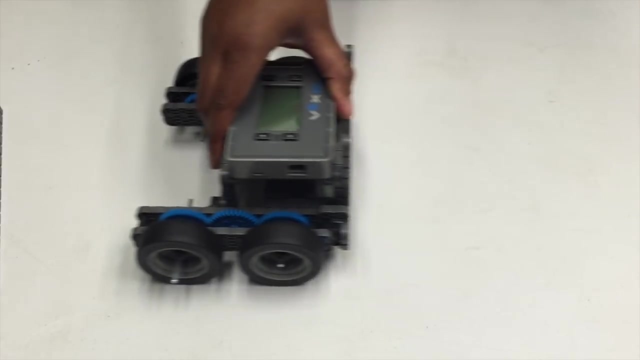 base around and notice you have two of the black corner connectors in the back that will need to connect to the 2 by 12 beam. Once you have those snapped in place, you have now completed your VEX IQ standard drive base. Now time to 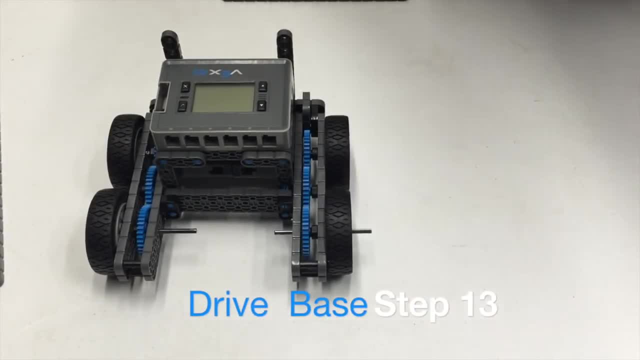 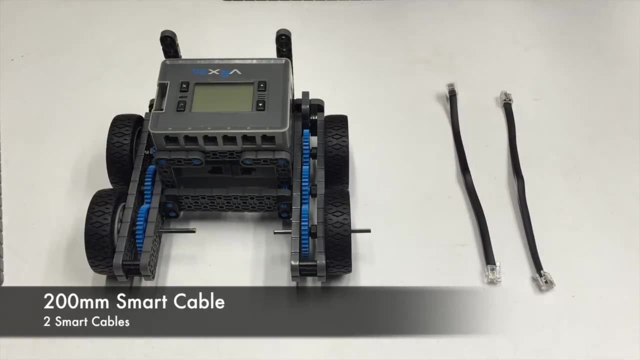 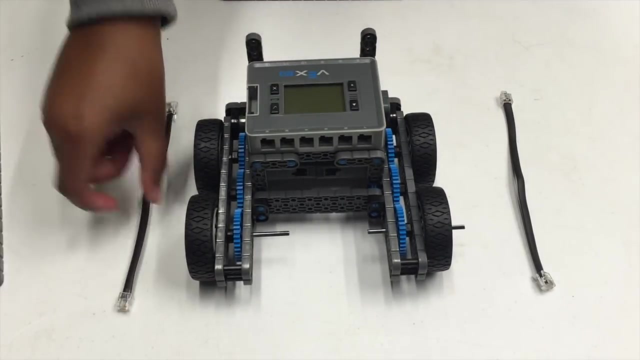 connect the cables: Step 13.. You will need two 200 millimeter smart cables. Partner A: you grab one of the smart cables and Partner B: you grab the other. You will need two 200 millimeter smart cables. You will need two 200 millimeter smart cables. 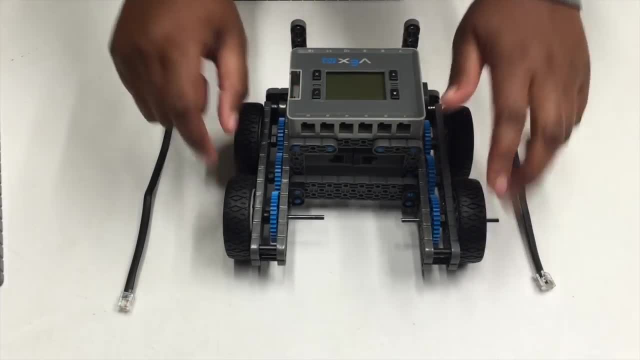 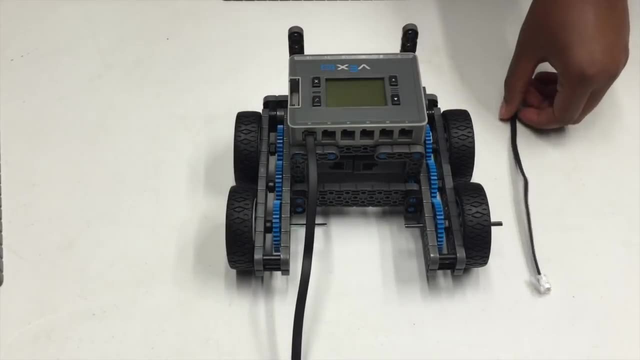 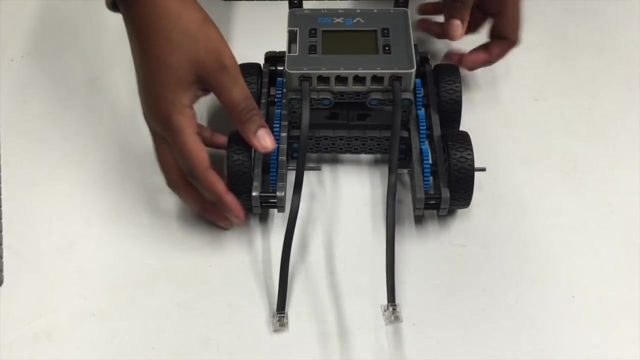 One of the cables will go into port 1, while the other will go into port 6.. Partner A, you put yours into port 6 first and then, Partner B, you put your cable into port 1.. The smart cables will connect underneath the VEX IQ robot. 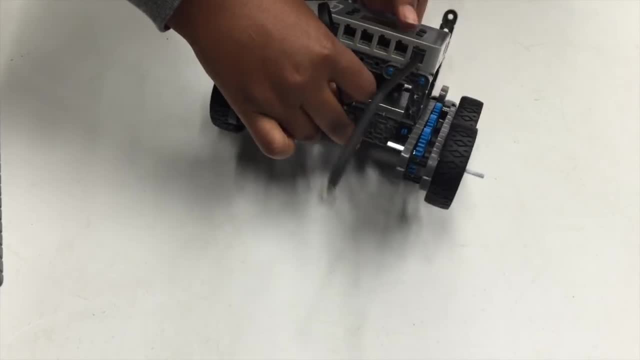 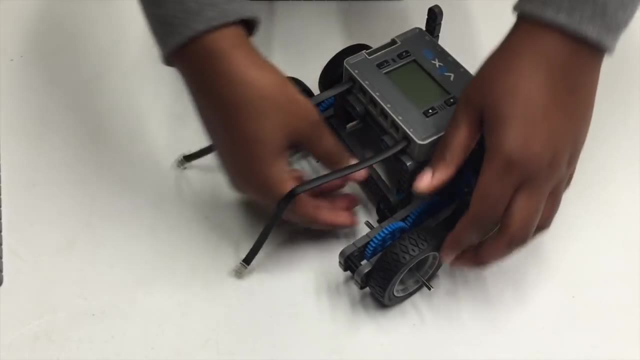 brain to the motors. Now, if you have fingers that are a little bit too large to fit in the space, you can do that by connecting the smart cables to the motor. You can detach your structure and then tuck the smart cable under to connect it to the 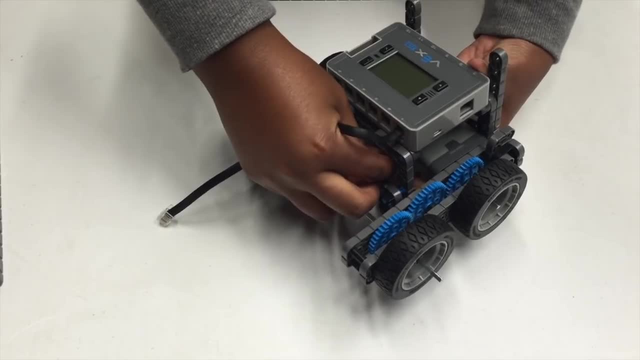 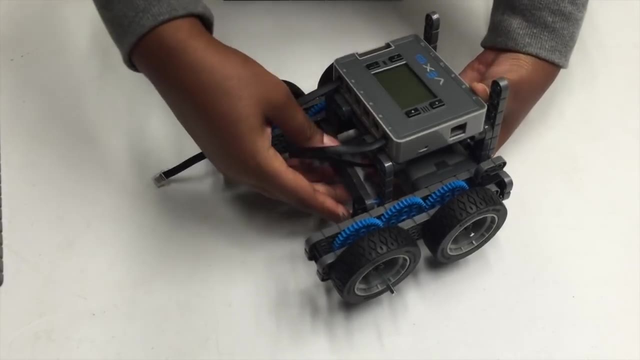 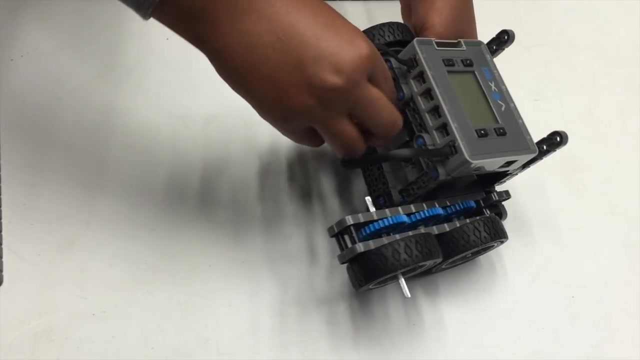 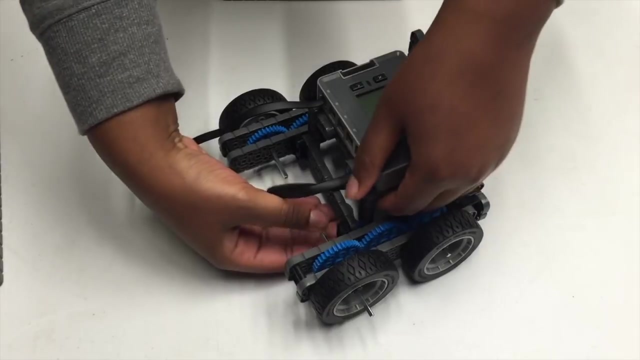 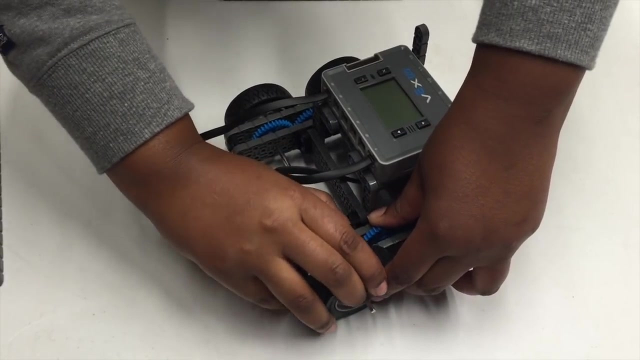 motors. This is not an easy step. It will take some time. so if you don't get on the first time, do not be discouraged. Just keep calm and build on. Once you get the first one on, go ahead and snap that one side back together and then. 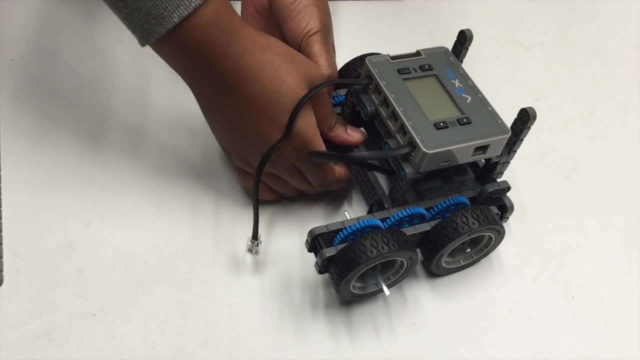 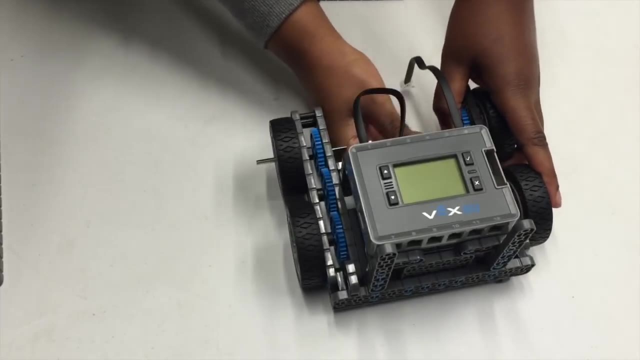 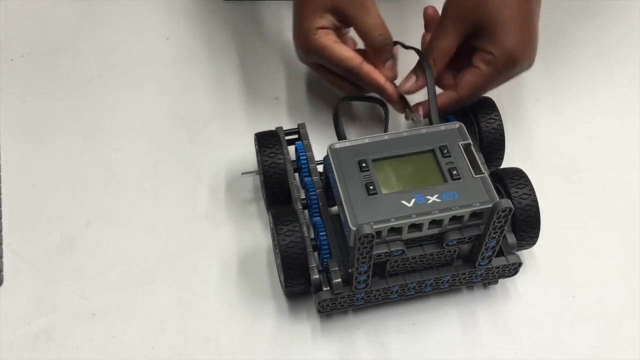 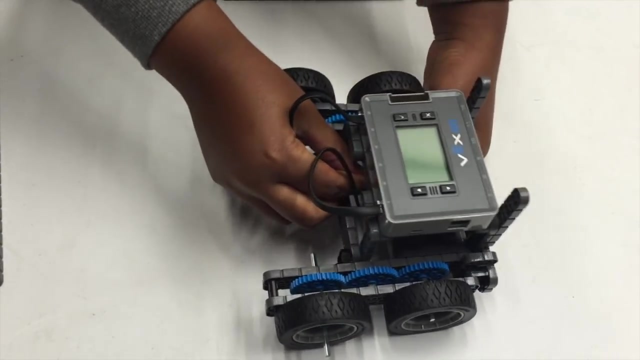 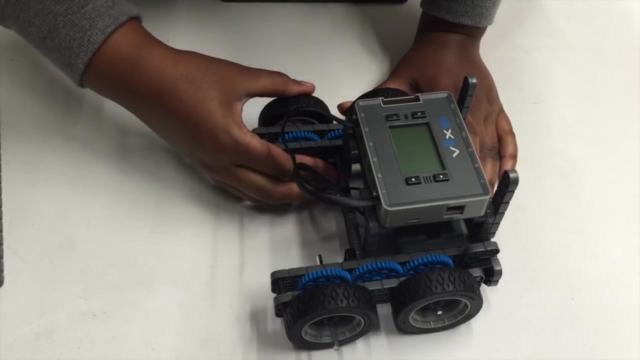 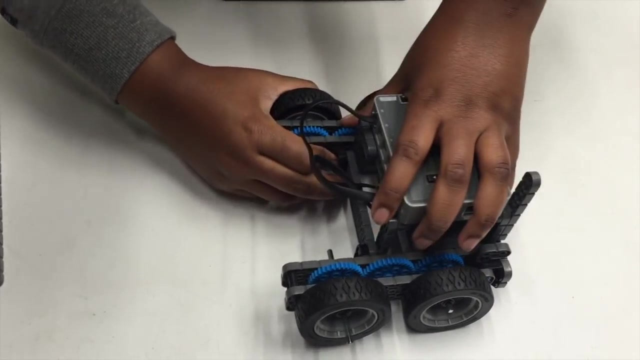 to get the other side. just detach the structure from the gears, and then you should be able to get the cable in the right spot. Again, be sure to take your time and not to pull too hard on the drive base There. Once it's in, go ahead and put your robot back together. 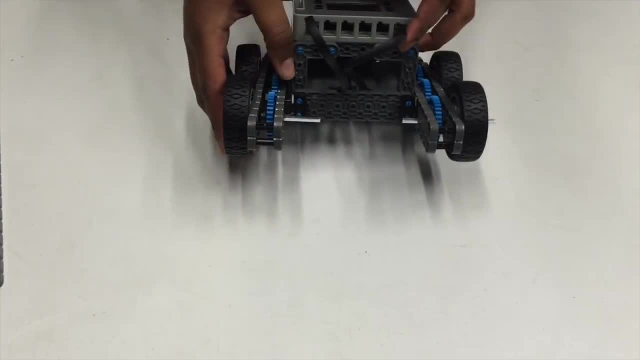 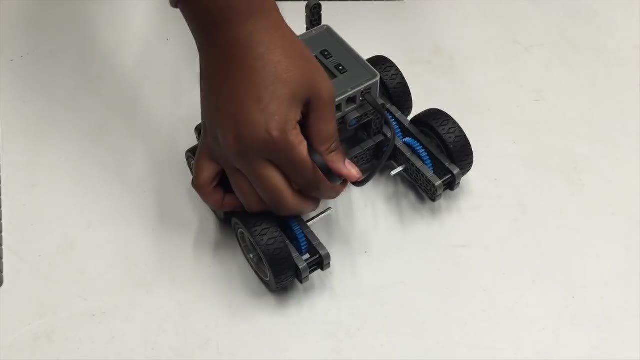 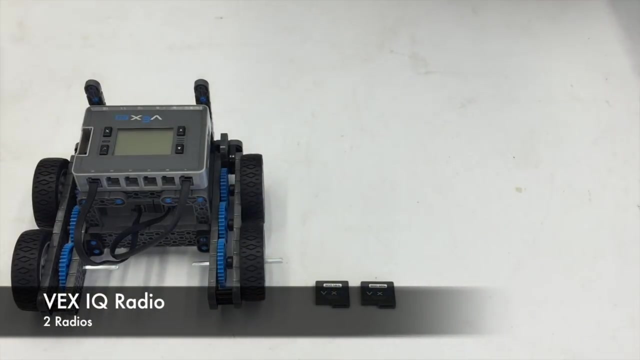 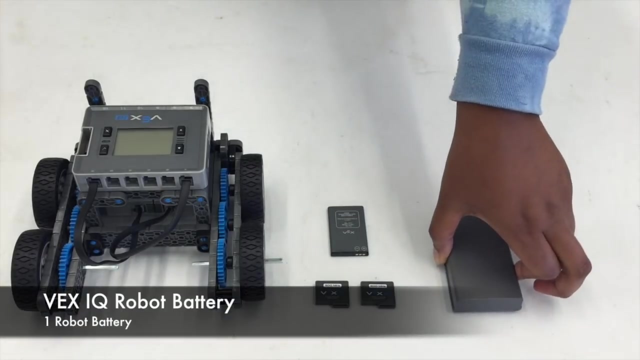 Again, the corner connectors go into the second hole from the shaft. now you're ready to connect your controllers. Step 14: you will need two VEX IQ radios, one VEX IQ controller battery, one VEX IQ robot battery and one. 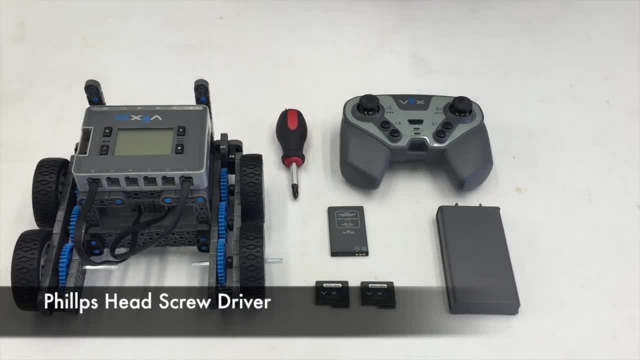 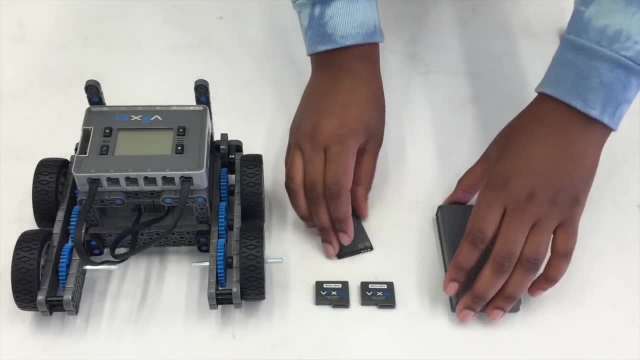 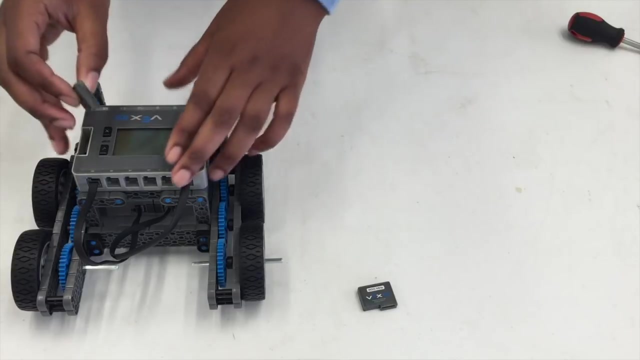 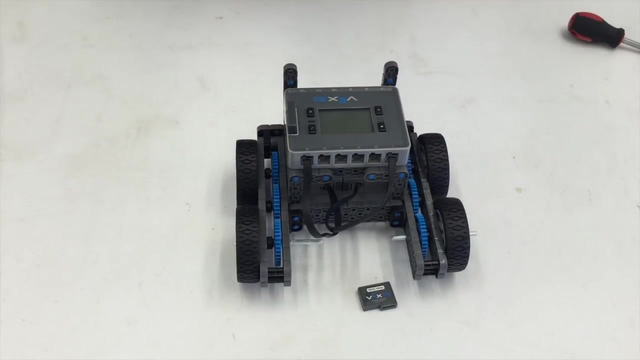 VEX IQ controller. You'll also need the Phillips head screwdriver to remove the casing from the back of the controller. One of the partners: grab one of the radios and place it into the open slot on top of the VEX IQ robot brain. Once that is done, grab your VEX IQ robot. 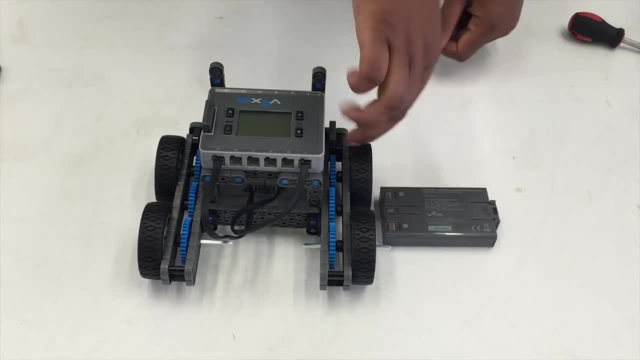 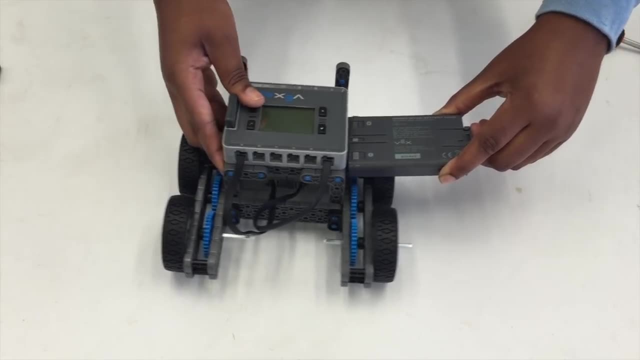 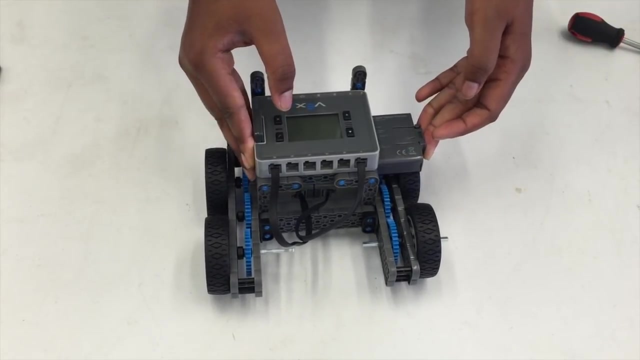 battery and you want to turn it upside down so that the words are facing up and you're going to slide it right underneath of the VEX IQ robot brain. You may have to remove the wheel. be sure not to jam it in there. just take your. 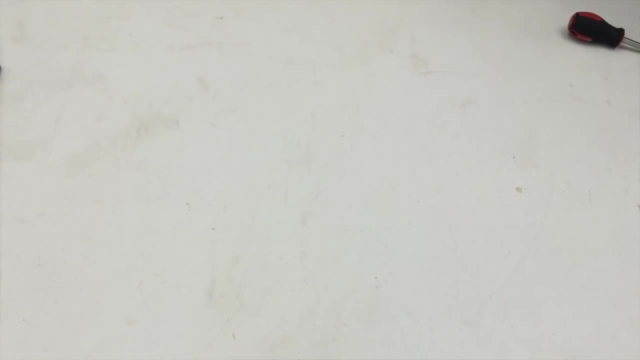 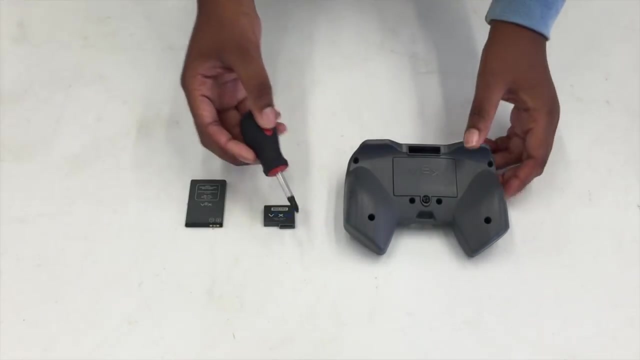 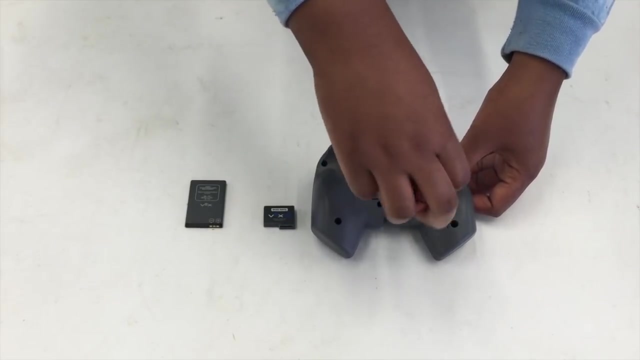 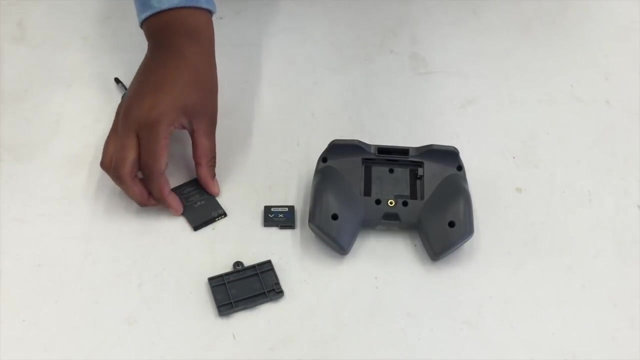 time and it will slide into place. Now grab your VEX IQ robot controller, one VEX IQ radio and one VEX IQ controller. Leap your VEX IQ robot with the receiver handed you. Once you get the VEX IQ robot case off, grab your VEX IQ controller battery and slide it in. 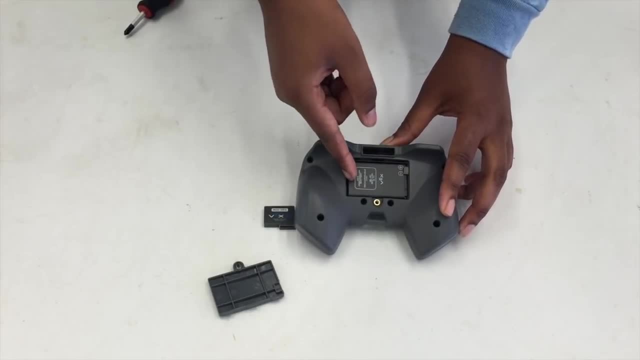 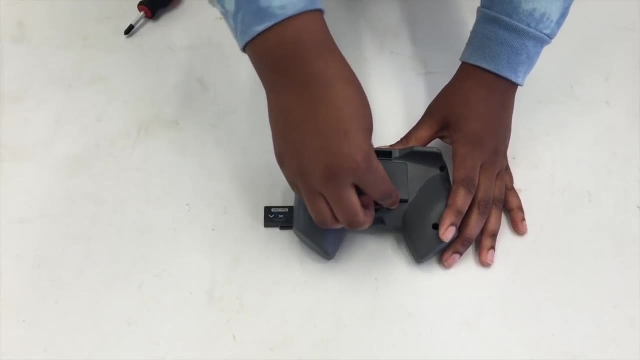 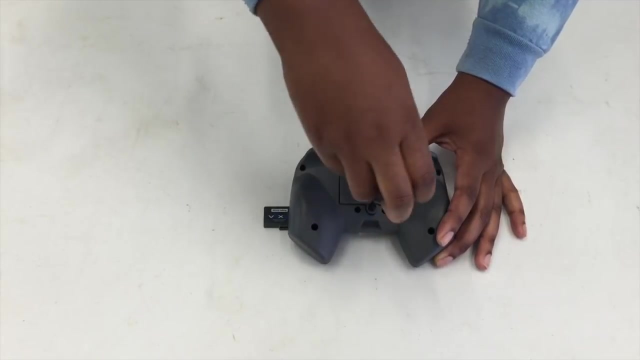 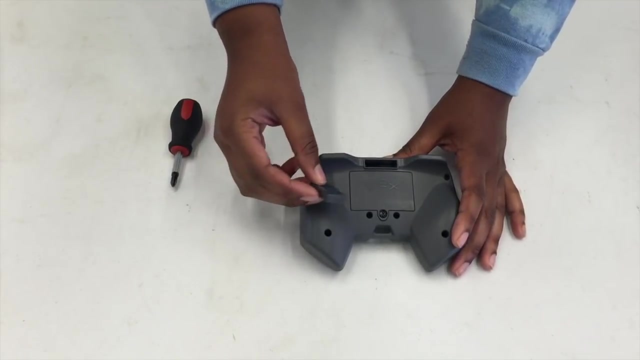 in so that the words are facing up. You can now place your case back on top and grab your screwdriver and screw it back in place. Once the case is tightened, you can grab your VAX IQ radio and place it in the slot in the 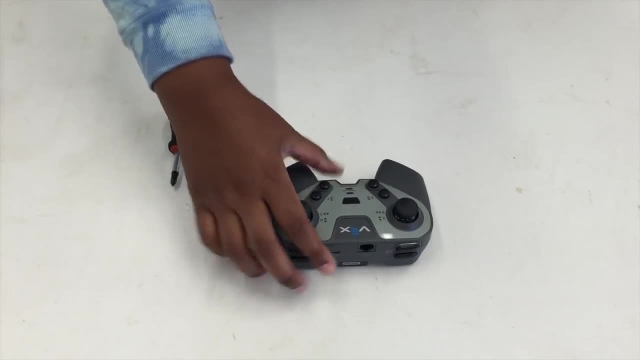 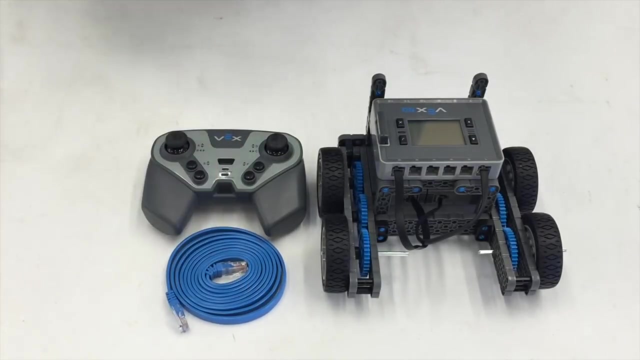 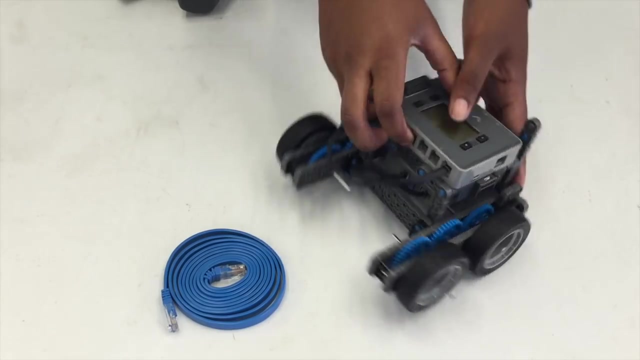 back of your VAX IQ controller. This last step is only for people who are just using your VEX iQ controller and they don't have a VEX iQ controller. So what? you using their VEX IQ set for the first time or, if, for some reason, your 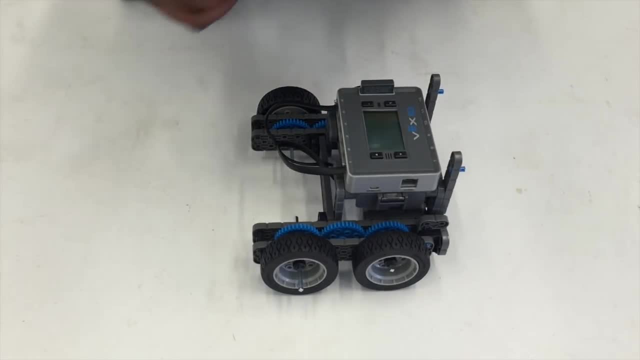 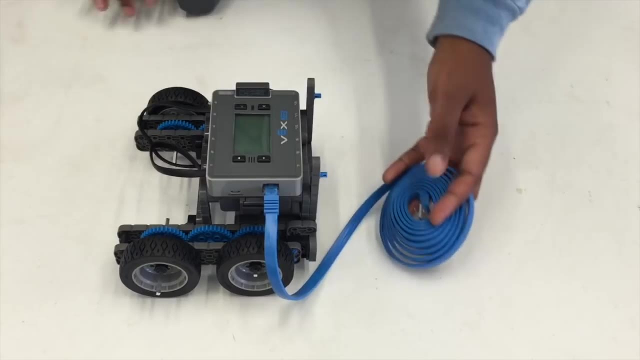 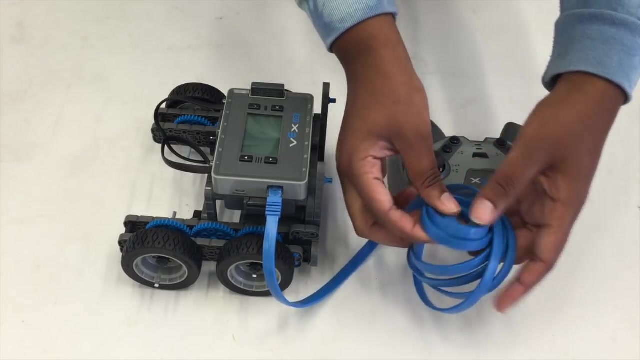 controllers aren't connected anymore. You will need the blue VEX IQ tether cable and you will plug it into the Ethernet port on the side of your VEX IQ brain. You will plug the other end of the VEX IQ tether cable into your controller.